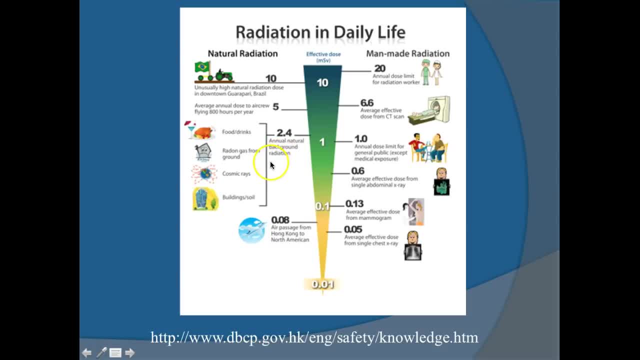 North America. there's some funny stuff in here, so there's natural here. so from food and drinks, like bananas have radiation in them right on. gas from the ground is a big exposure, especially people back east that have basements there's cosmic rays. and also from building and soils like bricks have they give off radiation. so 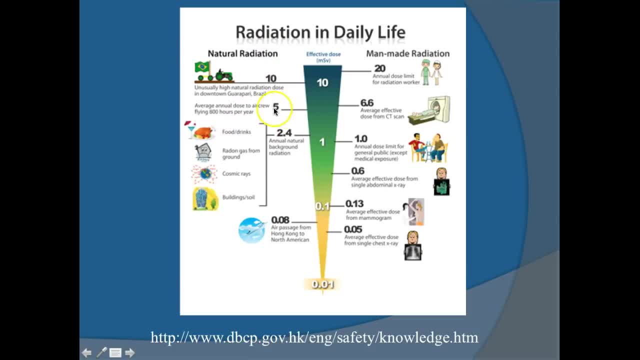 the annual dose to aircrew flying 800 hours. so they're here, so interesting, huh. and then radiation dose in downtown Brazil. so we look here in the man-made, we have a chest x-ray and we have a mammogram and an abdominal x-rays. you can see a little. 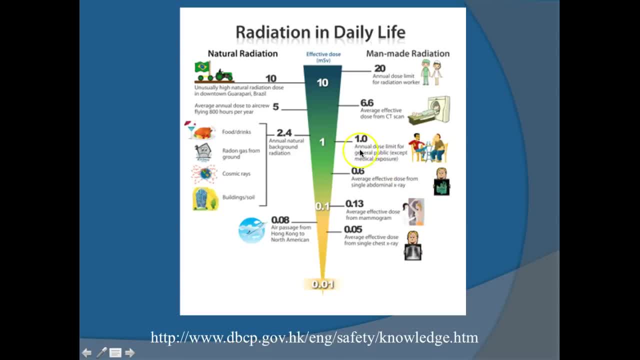 bit higher annual dose for the general public here, and then the average CT scan dose and then we have the radiation worker there. so background, so, like i said, you can get it from cosmic radiation, radioactive elements. radioactive elements are an Kalina for the common birch wood band. we have pressed filthy dust on the ground statue here. radioactive elements make CO2. it sor congregation. 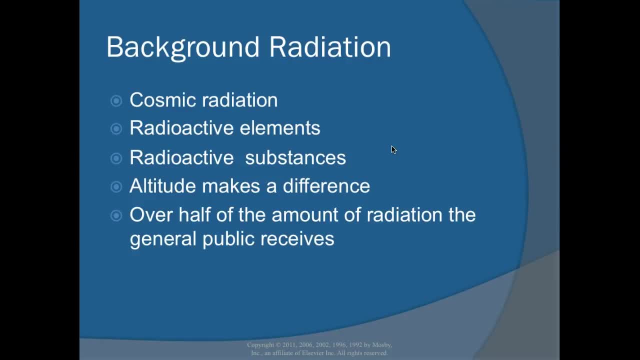 substances. altitude makes a big difference, so people living in Colorado are getting a lot more radiation than what we get here in San Diego, so over half the amount of the radiation to the general public. so we get radiation every day, all day, and depending on where we live and if we fly, a lot changes how. 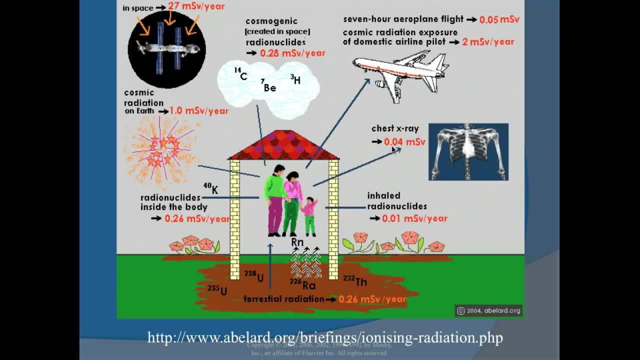 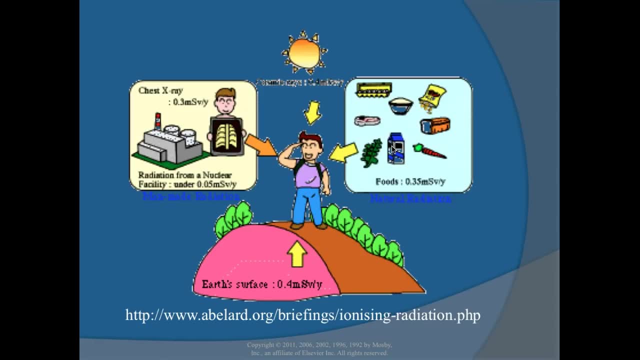 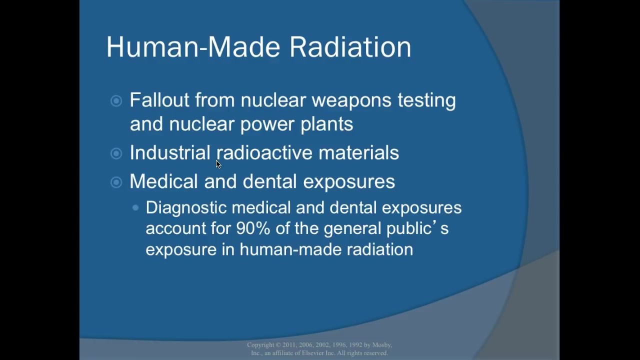 much radiation we receive and you can see. here's another graph for you help you understand where all the radiation is coming from. and here chest x-ray. and just from the soil we're receiving radon gas, and from the foods also- all right, man-made radiation. so there's fallout from nuclear weapons testing and nuclear. 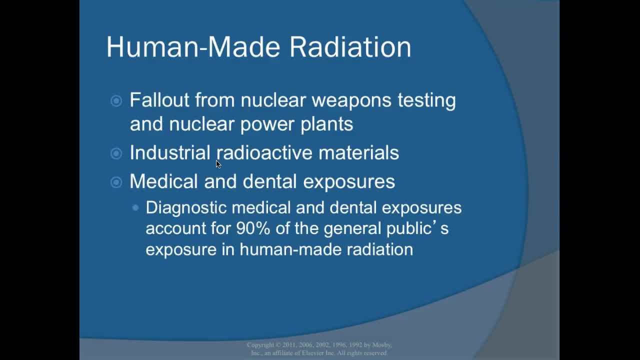 power plants. exciting how we know about Chernobyl. currently industrial radioactive materials also, so medical and dental exposures. this is the first time we've seen radiation from a nuclear power plant. this is where the diagnostic and medical exposures account for 90% of the general population's exposure, so it's considered man-made. oh then there's that. 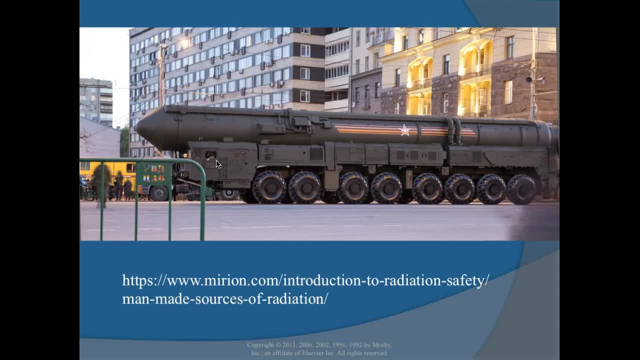 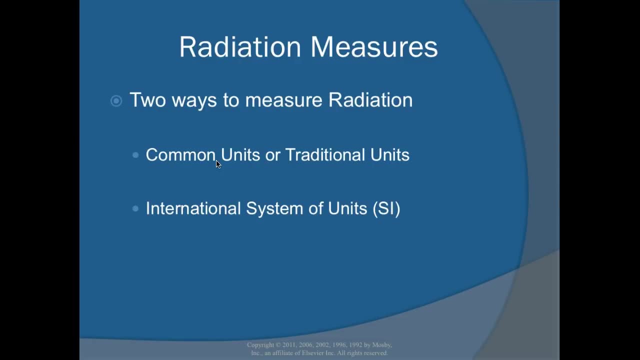 so that's a Russian nuclear bomb. very exciting to see that. all right radiation measures. now there's two different ways that we measure radiation. there's common units or traditional units, and there's the international units or the SI unit. it just happened that the ART just eliminated the common or traditional units. they 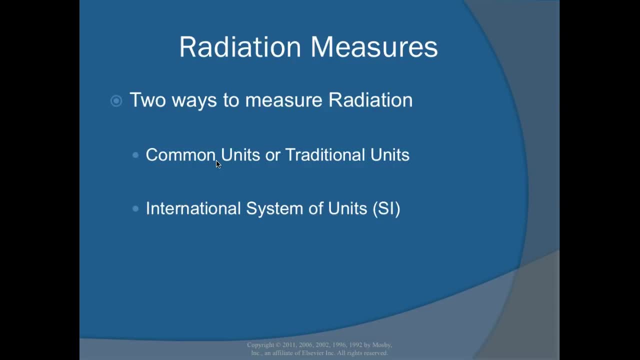 said that, starting 2017, they're not going to be asking you guys what the common or traditional units are on your national exam. the problem is, all of us here in the United States refer to it as common units or traditional units. so we are still going to make you know these common or traditional units and the SI. 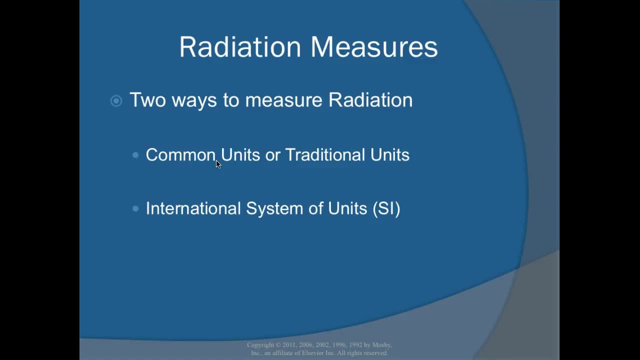 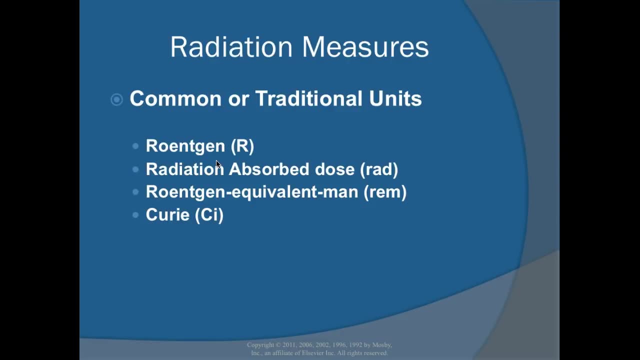 units in addition, so you will be able to relate to people in the clinic without just going to the SI units. alright, so with common or traditional units, we have the Rankin, which is the capital R. we have the radiation-absorbed dose, which is the rad. so each letter here. 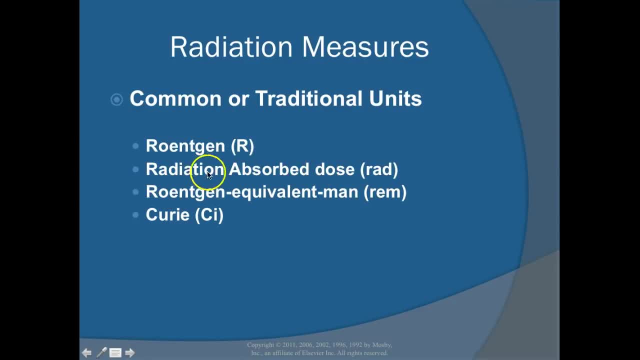 at the beginning are a D, the rad is radiation-absorbed dose, there's the Rankin equivalent, man, which is the REM, and we have the curry. so in the international system, which is the SI units, we have coulomb's dioxide, Coulombs per kilogram, Sieverts, Gray and Becquerel, and we'll compare the two. 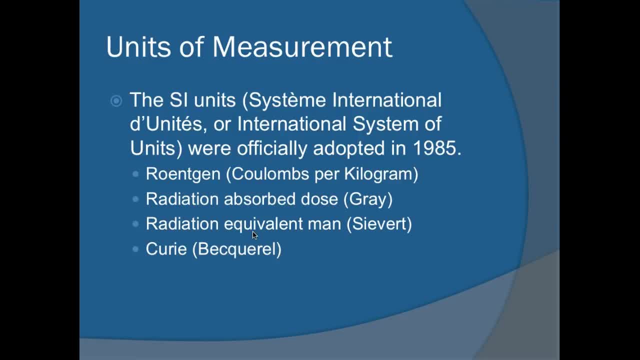 So the SI units were officially adopted in 1985, so we went from the Rankin to the Coulombs, per kilogram Radiation Absorbed Dose to the Gray and the Radiation Equivalent Mann, which is the REM, to the Sievert, and the Curie to the Becquerel. 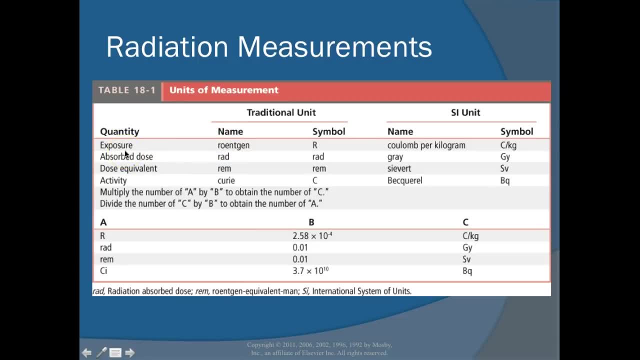 And you can see here. there's a graph. it's in one of your books, I think it's Bouchon. You have your exposure, which is measured in Rankin, which is the R and it's Coulombs per kilogram in the SI unit and it's the C over kg. 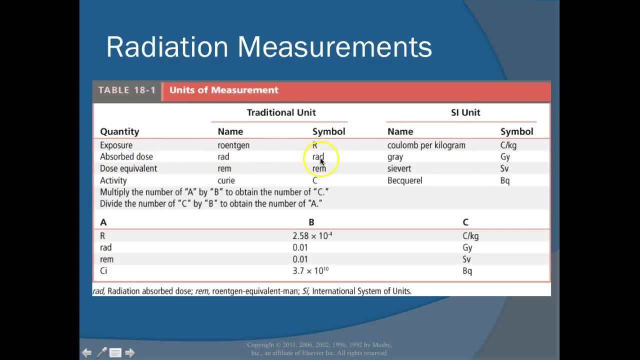 So the Absorbed Dose is the Rad, the Symbol is the Rad, and in the SI units is the Gray Dose Equivalent, which is the REM, and Symbol is the REM. And we have Sievert and then Activity is the Curie, with the C it's actually CI. 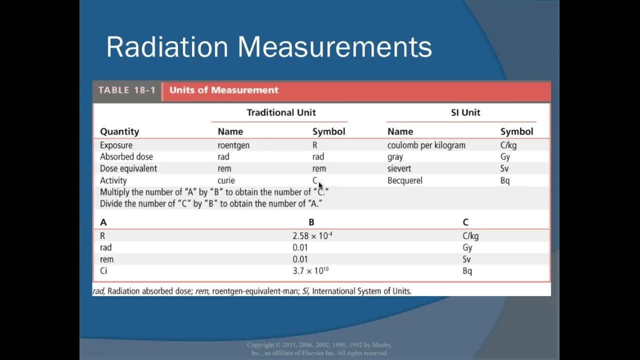 I don't know why they just have the C here. I guess it can go either way, but I haven't seen it without the I, so I think they missed it. I don't know. Anyway. and then there's the Becquerel, which is the BQ, and I'll give you a way to remember. 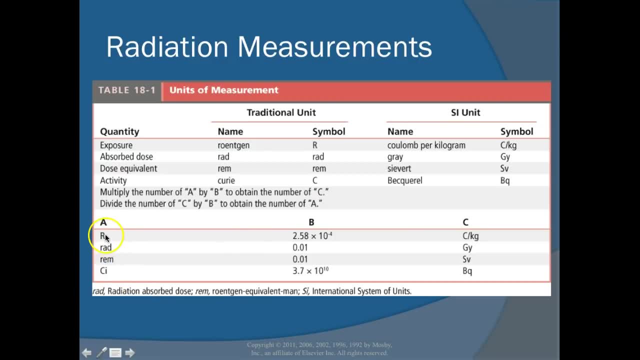 this a little bit easier So you can see the conversion here and the R. so if we look, multiply the number of A by B to obtain C, Divide the number of C to obtain B or to obtain the letter A. so here this is giving. 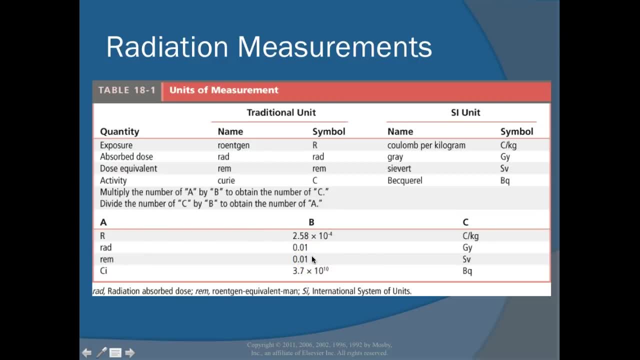 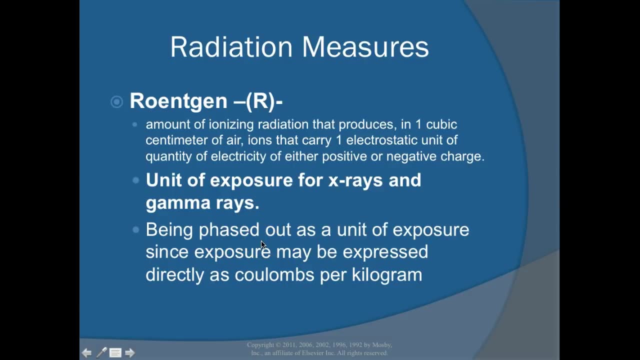 you the conversions for between the traditional and the SI units. Okay, so the Rankine, what is it? So this is the amount of ionizing radiation that produces in one cubic centimeter of air- Air is your key word there: air ions that carry one electrostatic unit of quantity of. 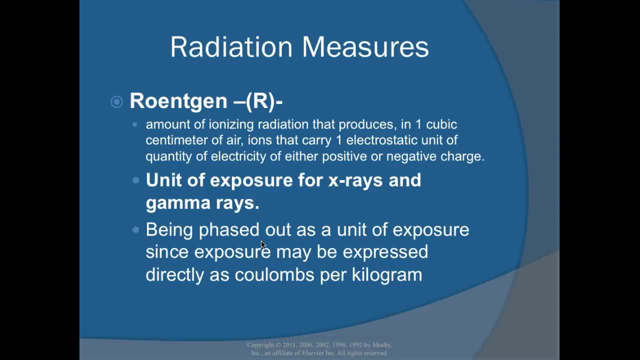 electricity, either positive or negative, So it's ionizing radiation in air is what you're looking for for the definition there. So the unit of exposure for X-rays and gamma rays. so we use the Rankine for diagnostic levels here within radiology and it's being phased out as a unit of exposure, since exposure 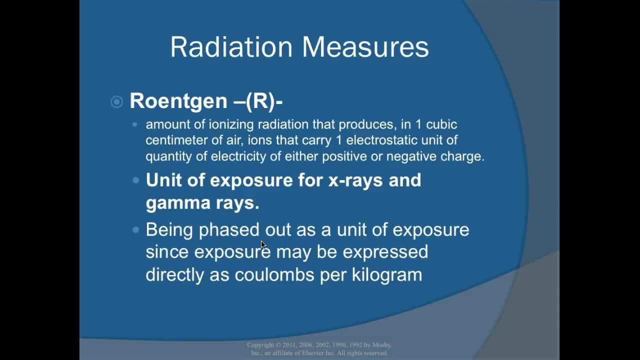 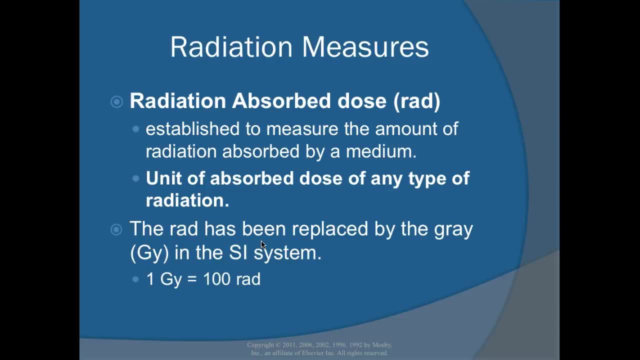 may be expressed directly as coulombs per kilogram, which is the SI unit. There's the radiation-absorbed dose, which is the RAD. it's established to measure the amount of radiation absorbed by a medium. So if we're talking about how much dose did the patient receive, we're talking about the 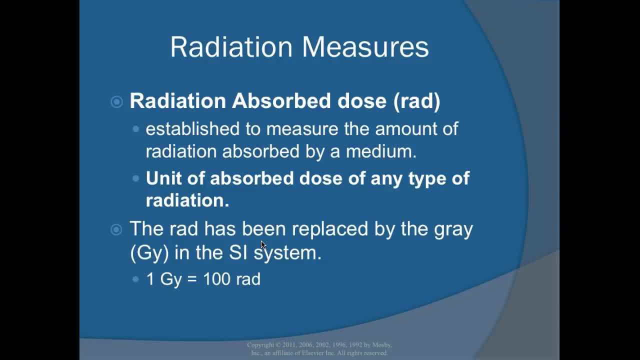 RAD, okay, So it's unit of absorbed dose of any type of radiation. so the radiation, the RAD, has been replaced by the gray in the SI unit, So one gray is 100 RADs. so it's not a direct conversion, it's not a one-to-one, it's a 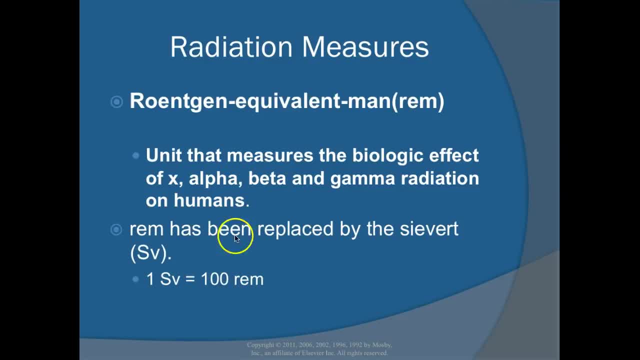 one-to-100.. The Rankine equivalent man or the REM. so you got the R, the E and the M. So the REM is a unit that measures the biological effect of X-ray alpha beta gamma radiation in humans. 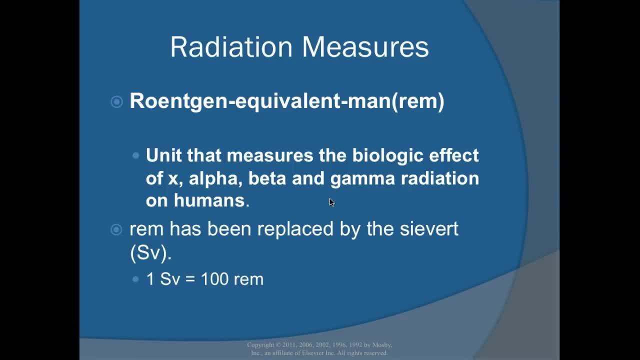 So the REM has been replaced by the SIVRT. So this is the amount of radiation to see changes within the body. So all of our dose badges are measured in REM. So this is the unit that measures biological effects. Oh, and one SIVRT equals 100 REM. 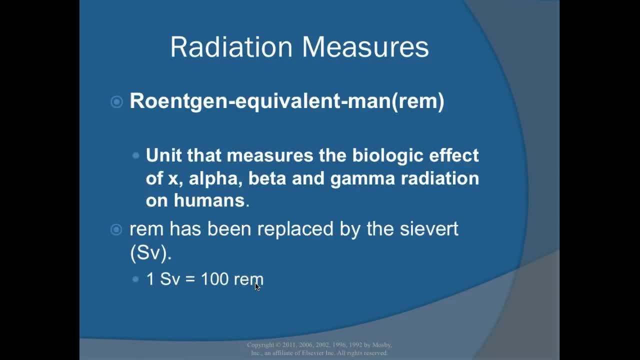 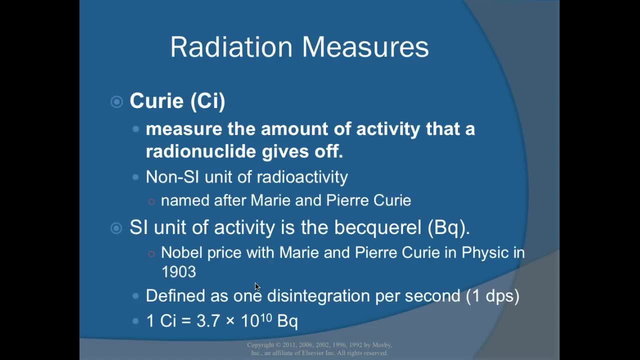 So, just like with the RAD and the gray, so we're dealing with the same thing here, So it's a one-to-100.. The CURRIE, It is the measure, measures the amount of activity that a radionuclide gives off. 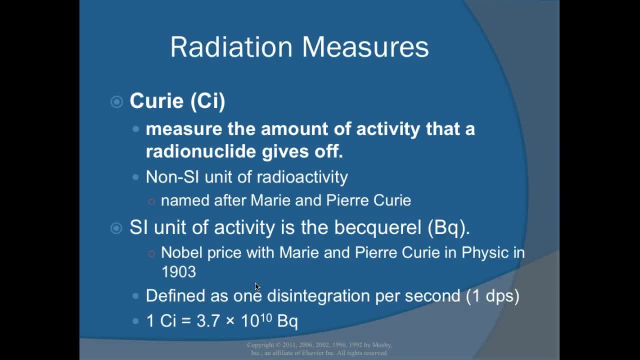 So a non-SI unit of activity. It's named after Marie and Puri CURRIE, So Marie CURRIE- as you guys have learned over the summer, she is the person that started up a bunch of mobile X-rays. Okay, 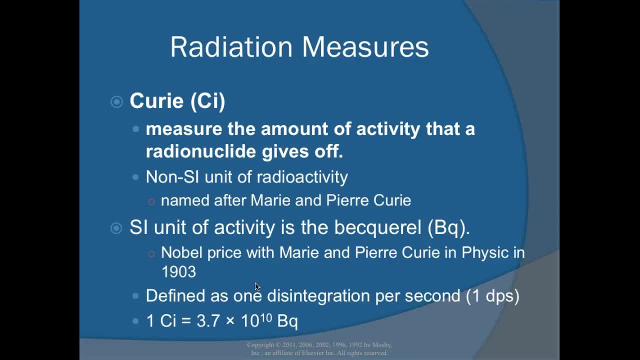 She also did a bunch of research on radium and refinement and Puri and well, she got a Nobel Prize. And then her Puri, her husband and Henry Becquerel received the Nobel Prize in physics in 1903. So the three of them got a Nobel Prize in physics in 1903.. 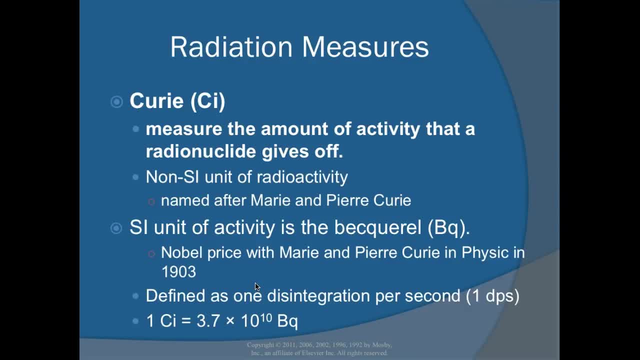 So Marie CURRIE, or Marie and Puri CURRIE, is the traditional units, So they're traditional, They're married, They're traditional. Becquerel is in the SI units, So he got the Nobel Prize with all three of them, but he was left out of the marriage. 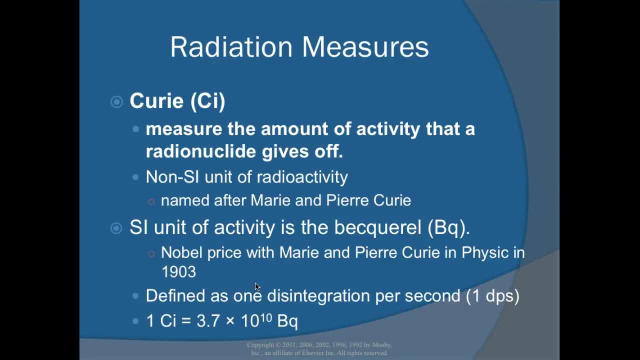 That's how I remember it. So the traditional units: they're married, Marie and Puri, they're traditionally married. And then you have the SI unit, which is Becquerel. Okay, I don't know if that helps you remember it, but it did me. 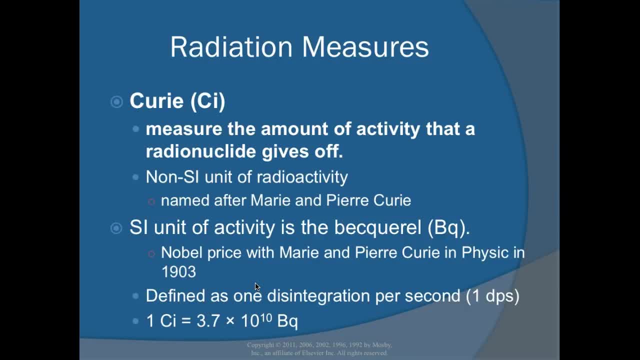 So it's defined as one disintegration per second. So the CI is equal to 3.7 times 10.5.. Okay, So the CI is equal to 3.7 times 10.5 times 10 to the 10th Becquerels. 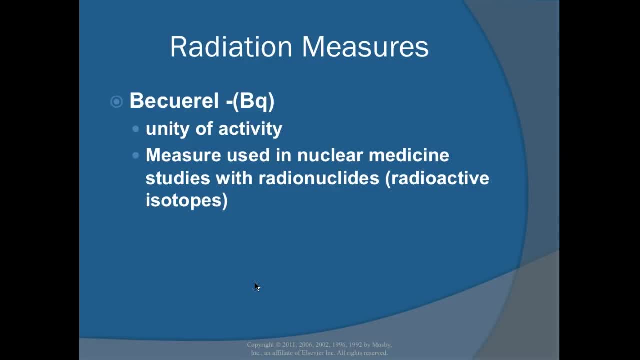 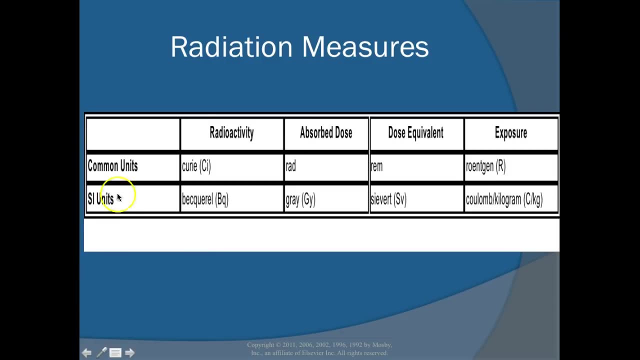 That's an easy conversion. All right, So Becquerel is the unit activity measured in nuclear medicine studies with radionuclides. All right, Here's another graph for you. So this is radiation measures. We have radioactivity absorbed dose and dose equivalent. 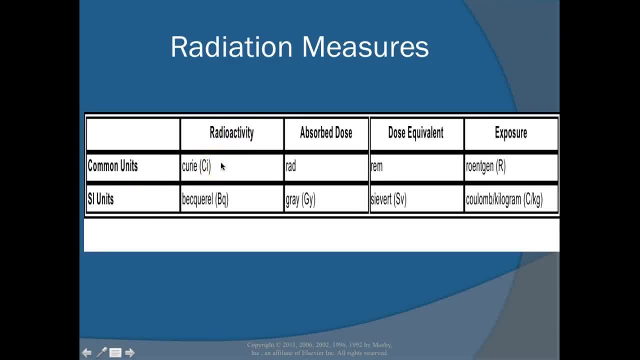 So we have the common units, SI, So radioactivity, we have the CURRIE, See the CI. The CURRIE for radioactivity and SI units is the Becquerel. So in common units we have absorbed dose, which is the rad. 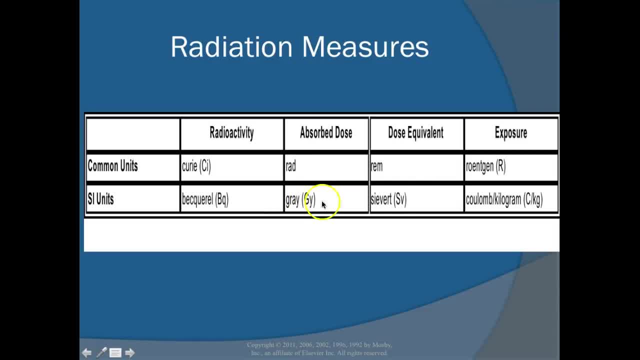 And in SI units it's the gray, And here we have dose equivalent, which is the rem, And then we have the SI units of Sievert. So remember, it's a one to 100.. So this is one, These are, 100 is the conversion. 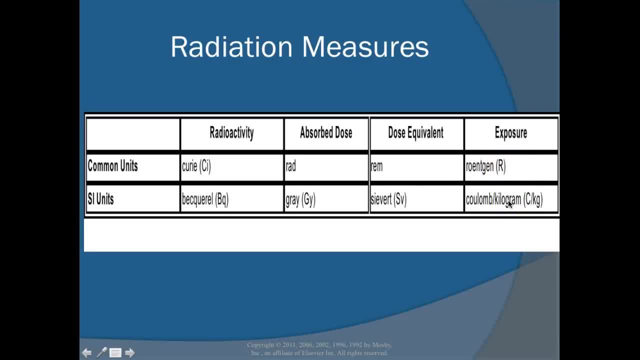 And then you have exposure, You have the Rankin and it's coulombs per kilogram. So this is backwards in the way that I presented it. It's kind of good because it shows you out of order. So you just have to memorize this stuff, you guys. 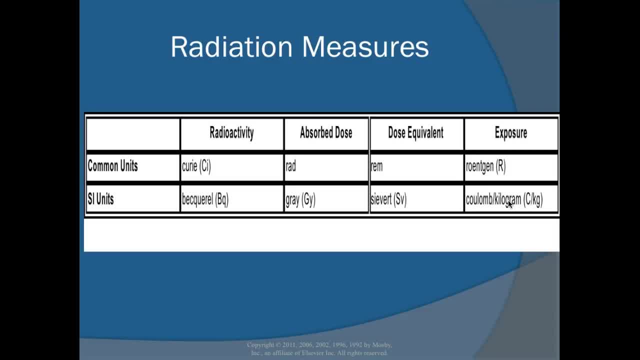 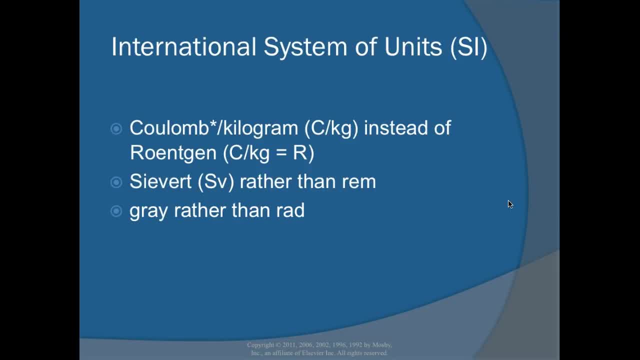 You're going to have to know both. I'm sorry, I'm going to just switch to SI units. You have to know both because no one in clinic really knows the SI units. All right, So here it is again. review: The SI units is coulombs per kilogram instead of the Rankin. 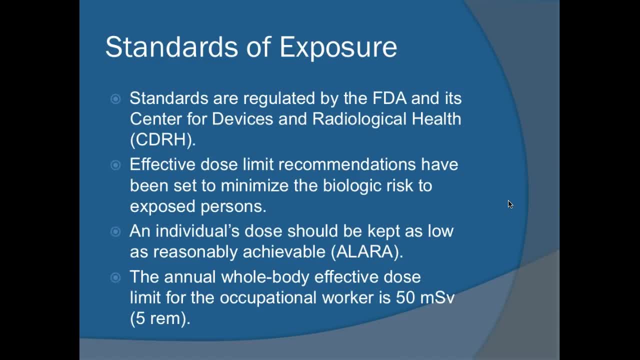 Sieverts rather than the rem, and the gray rather than the rad. So standards of exposure Standards are regulated by the FDA and it's Center for Devices and Radiologic Health. Hold on, OK. Effective dose limits: Recommendations have been set to minimize the biological risk. 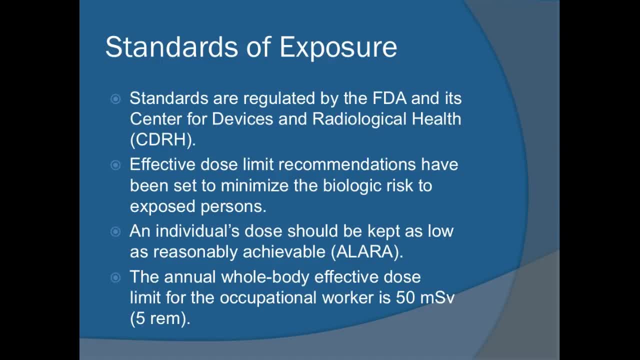 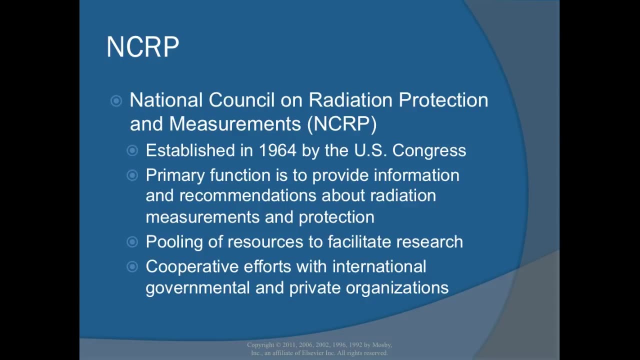 to exposed persons. An individual's dose should be kept as low as reasonably achievable. so a LARA, The annual whole body effective dose for a limit for the occupational worker, is 50 millisieverts or 5 rem. So the NCRP is a National Council on Radiation Protection. 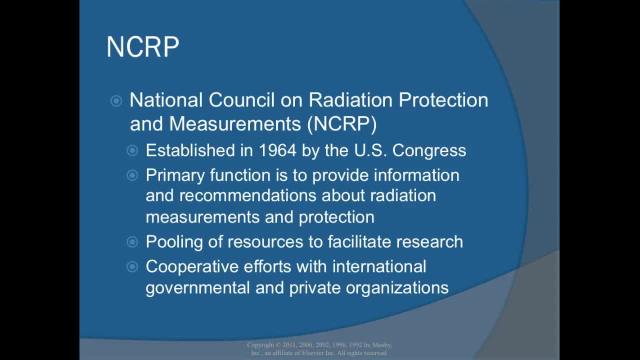 and Measures. It's established in 1964 by Congress. Its primary function is to provide information and recommendations, measures and protections, pulling of resources to facilitate research and cooperative effects efforts in international government organizations. so having everyone work together. so the goal, the primary goal, is keep radiation. 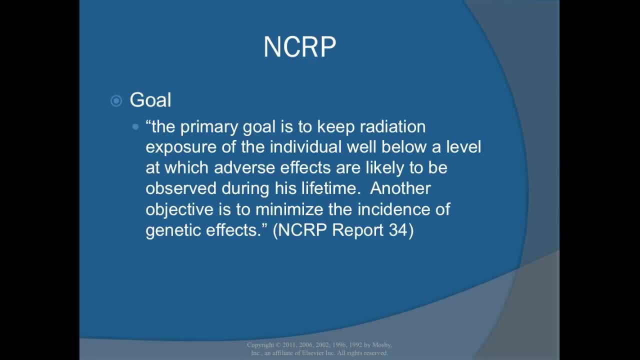 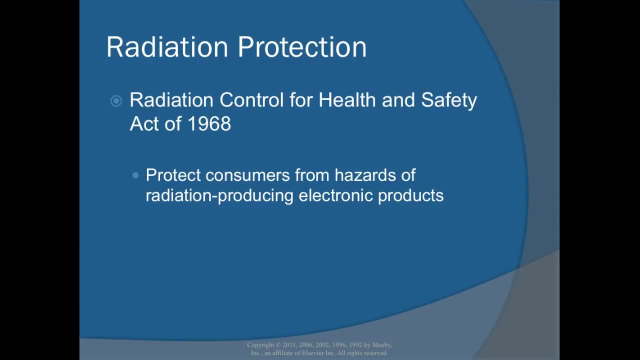 exposure to the individual well below the level at which adverse effects likely to be observed during his or her lifetime. another objective is to minimize the incident of genetic effects. so you will need to know what the NCRP goal is: radiation protection, so the radiation control for Health and Safety. 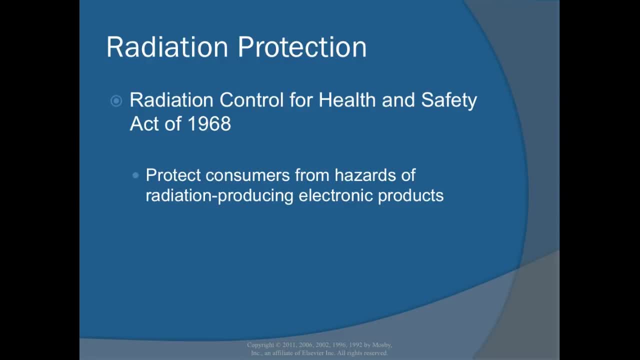 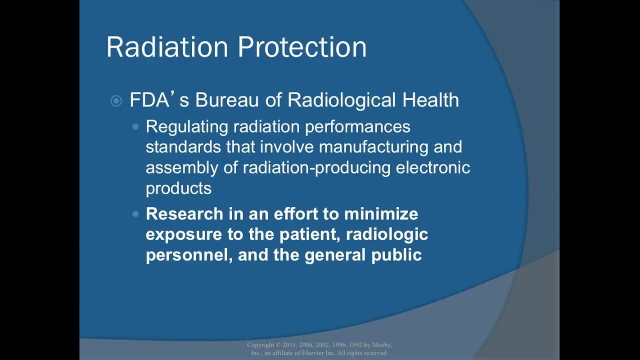 Act of 1968. it protects customers from hazards of radiation producing electric electronic products and the FDA's Bureau of radiologic health. so it regulates radiation performance standards that involve manufacturing and assembly of radiation producing elements, electronic device, so research in an effort to minimize exposure to the 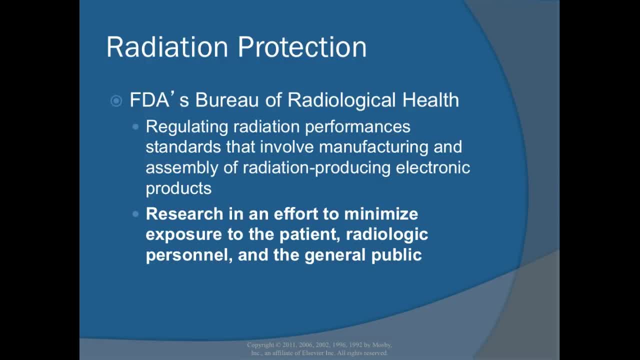 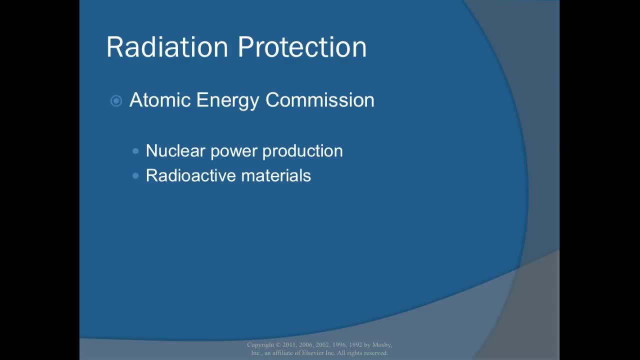 patient, radiologic personnel and the general public. the Atomic Energy Commission, so they oversee the nuclear power production and they manage the radioactive materials. the EPA, so the Environmental Protection Agency, environmental radiologic health protection, so they oversee generally everything going on if there's a big, huge radioactive spill. the EPA's. 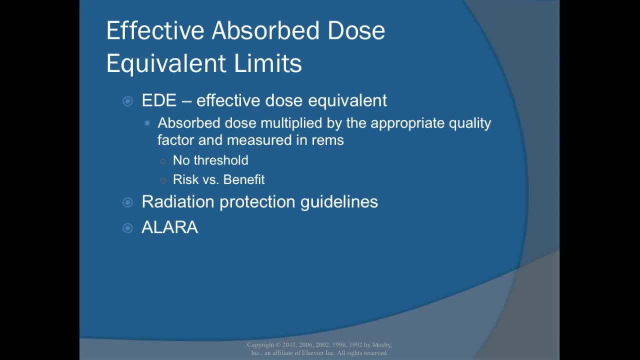 clearly is going to get involved. so effective absorbed dose equivalent limits. so the E D E is the effective dose equivalent. effective dose equivalent so the absorbed dose multiplied by the appropriate quality factor and measured in rems. so there's. the idea of this thing is that there's no threshold and 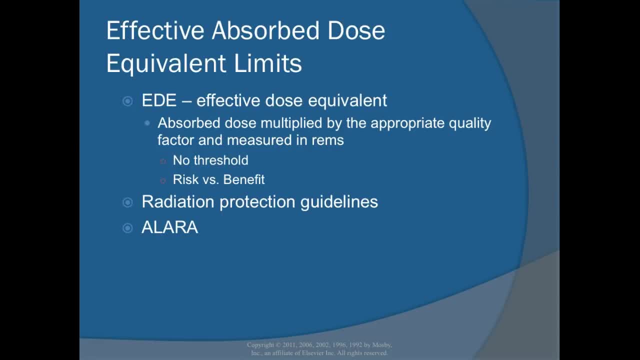 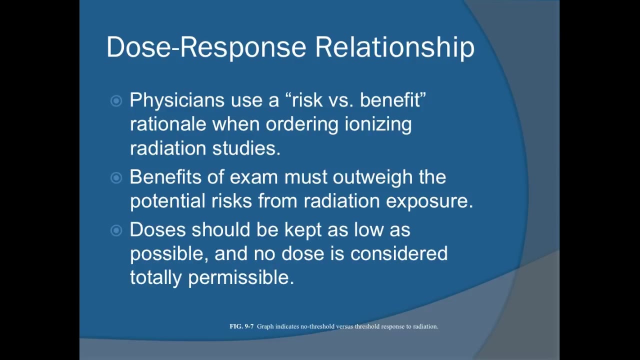 we look at the risk versus the benefits. so basic action, so the radiation control for health. it has原代, basically the radiation guidelines, and we go by a Laura trying to keep all this down, all the radiation. okay, so the ED is your effective dose equivalent and your 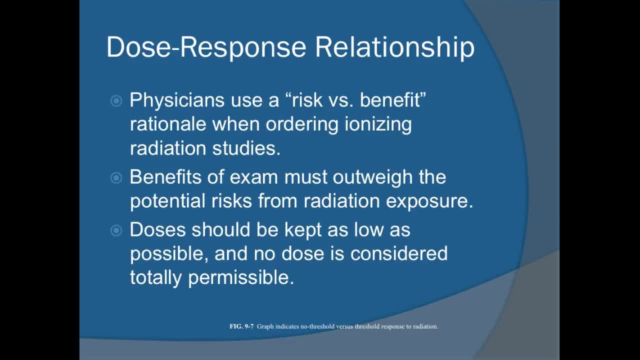 dose-response relationship, so the physicians should use a risk versus benefit rationale ordering radiation studies and the benefit of the exam must outweigh the risk of the radiation exposure and doses should be kept as dose is considered totally permissible- totally. it's important to know that we are working with a non threshold, so any amount of radiation can cause biological 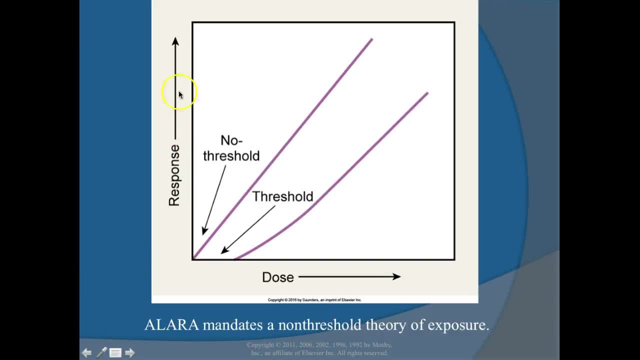 effects. so, looking here, this is the response to the body and this is the dose. so, as you can see, non threshold is here, it's coming, showing that any dose is going to cause a biological effect. not or a threshold shows that there's an amount of radiation that the body would be able to handle before there's 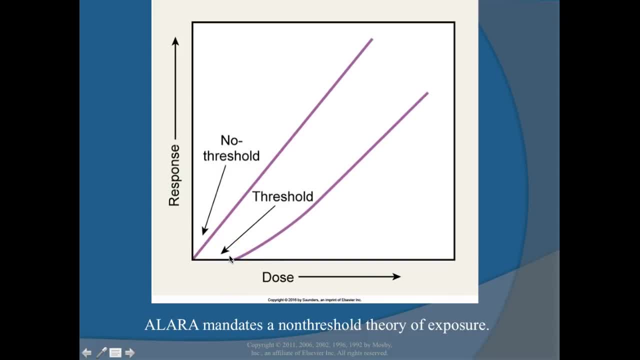 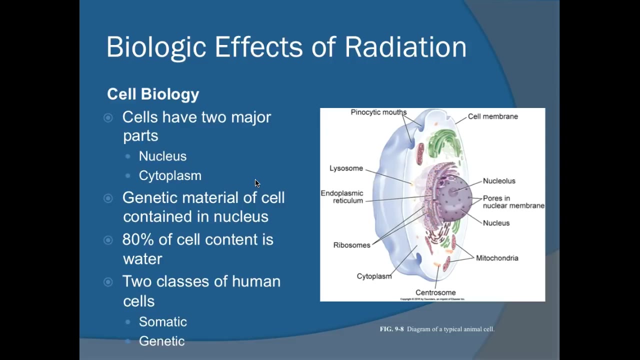 biological changes. so when we work in radiation we go off of the factor that there is no threshold, so any amount can cause damage, biological damage. so when we talk about biological effects of radiation, so you have to look at the cell biology. so they have two main parts: there's the nucleus and the cytoplasm, the genetic. 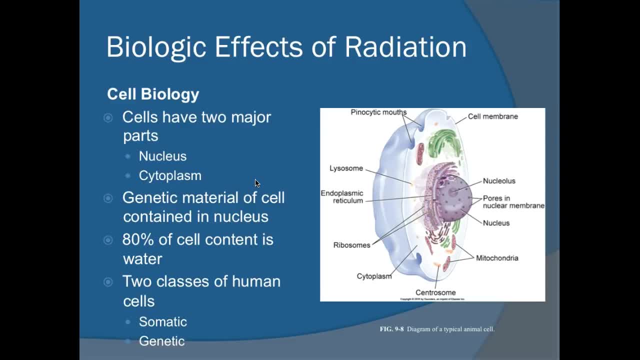 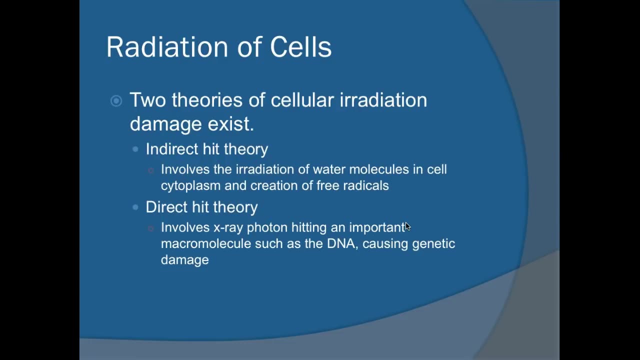 material of the cell is contained within the nucleus, so eighty percent of the cell is water. then the two classes of human cells are somatic and genetic. so if you don't remember what a cell looks like, this is what the cell looks like. so there's two theories of cellular irradiation damage. so there's direct and 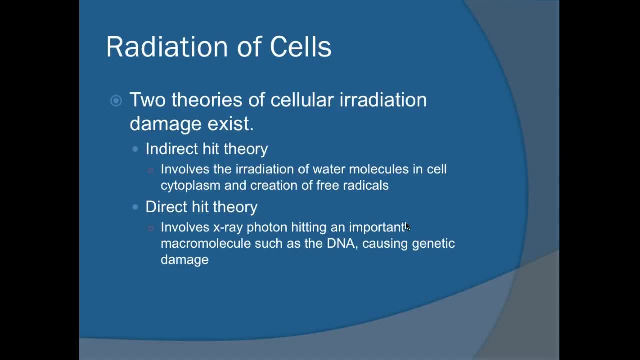 indirect hit theories. so the direct involves the irradiation of water molecules in cell cytoplasm and creates free radicals. so the direct hit method involves x-ray photons hitting an important area such as the DNA, causing genetic damage. so the indirect method just kind of causes free radicals within. 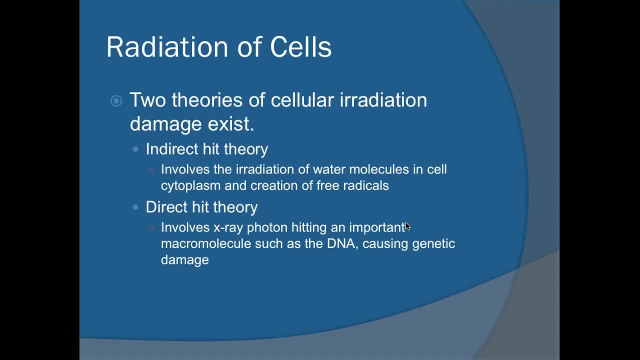 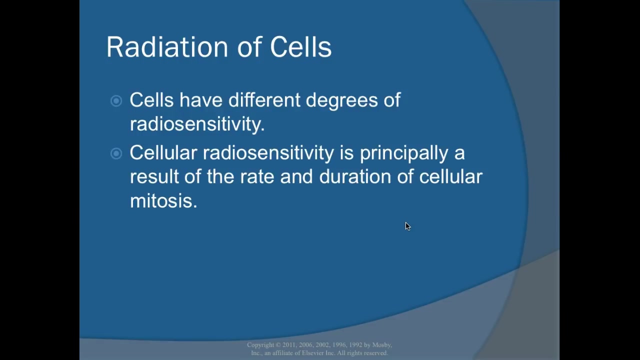 the cell so it can change the cell may not. it may be able to heal and recover. where the direct hit hits the DNA and changes the cell, damages the cell could kill the cell or it could reproduce as a different genetic type. so cancer radiation of cells. cells have different degrees of radio sensitivity, so cellular 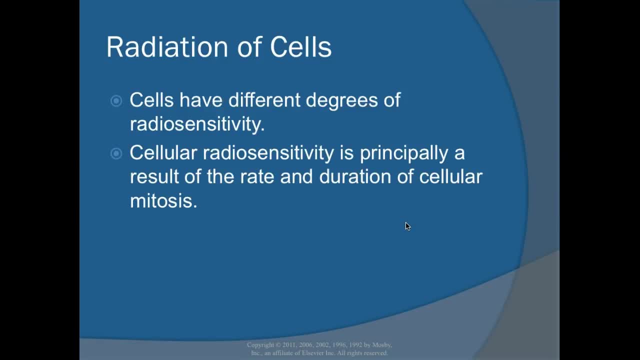 radius and sensitivity is principally a result of the rate and duration of the cell mitosis. so we talk about the division of cells. so when we are looking at our life stages, so if we look at a fetus who is growing rapidly, that's where we're looking, that that is the most sensitive. so where, as an adult, 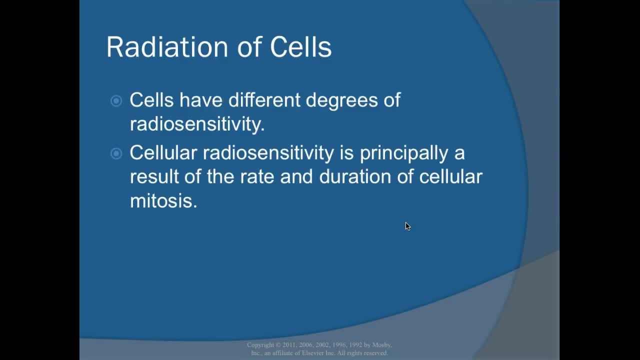 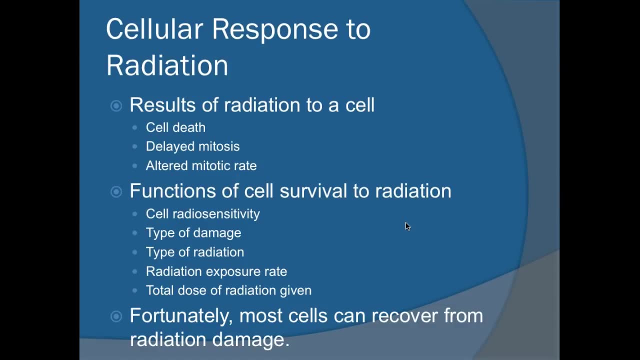 nerve cells are don't change. they're the most radio and resistant. so cellular response to radiation, so results of radiation to a cell. so this can happen when radiation is when a person is exposed, the cell can die, it can delay mitosis and it can alter the my mitotic rate. so 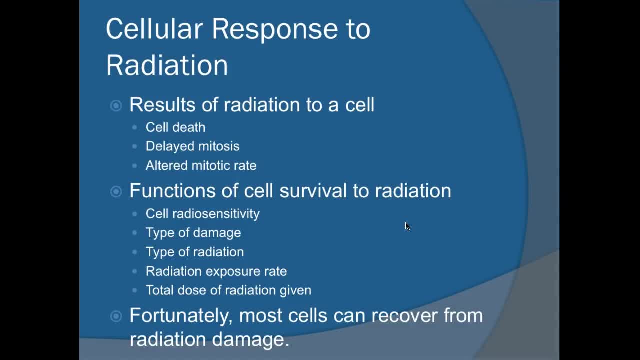 functions of the cell survival to radiation. so functions, as of cell survival to radiation. so cells radio sensitivity. so some cells, like the lining of our gut, is really sensitive, whereas our nerves are not. so cell radio sensitivity: we got to look at the type of damage that happened, the type of 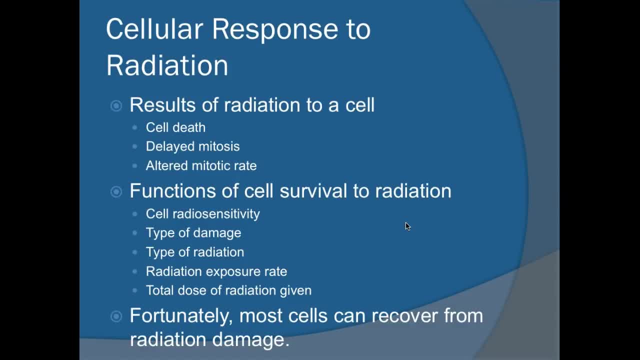 radiation that they received. there's a big difference between x-rays versus an alpha particle within the body and radiation exposure- radiation exposure. so how did our cells react when radiation was released, went through radiation, and how much radiation did they get from radiation, and how much radiation did they get, what rate? how long were they exposed, into what dose? 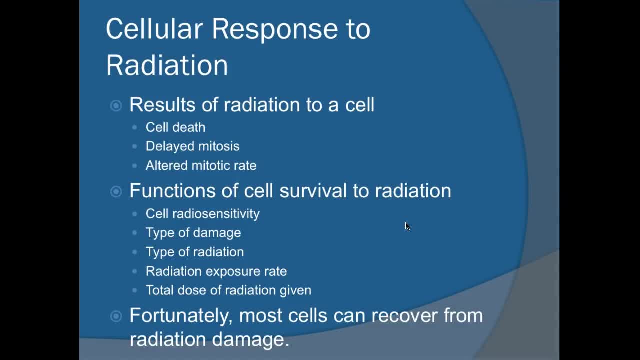 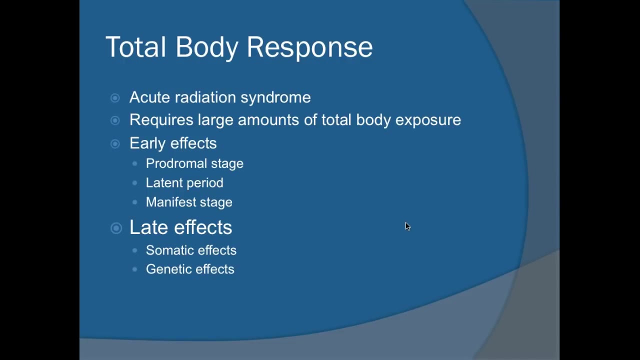 were they exposed. so the total dose of radiation given. if you're really interested in all this we're going to. we're going to cover it again when we get to fluoroscopy and this is covered a lot if you go into radiation therapy. fortunately, most cells can recover from radiation damage from diagnostic imaging. 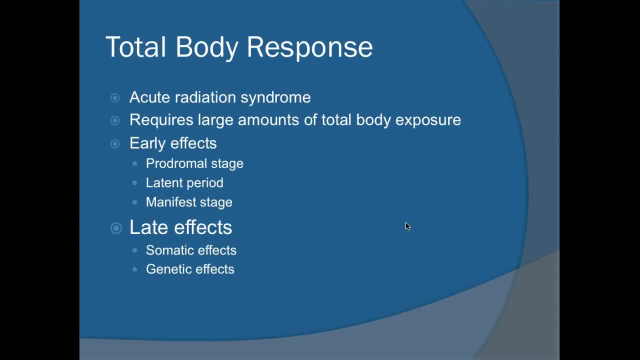 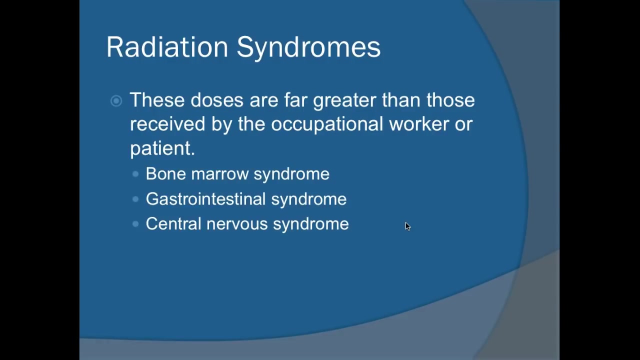 of total body exposure. so early effects: you have a perdomal stage, latent period and then it goes to manifest and then you have late effects. you have somatic and genetic changes which are not good, radiation syndromes. like I said, if we're just gonna brush over it, because we're gonna go really deep into this in floral 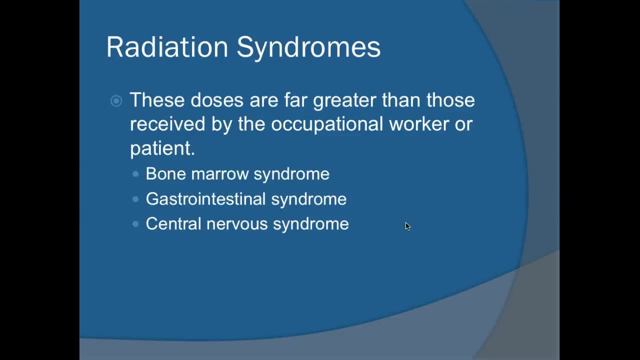 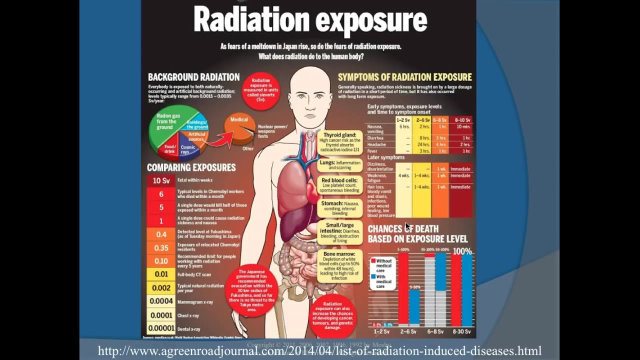 so these doses are far greater than those received by the occupational worker or the patient. so we can look at bone marrow syndrome, gastrointestinal syndrome and central nervous syndrome. so there's different things that happen with doses of radiation. so when we look at the radiation exposure, this is a 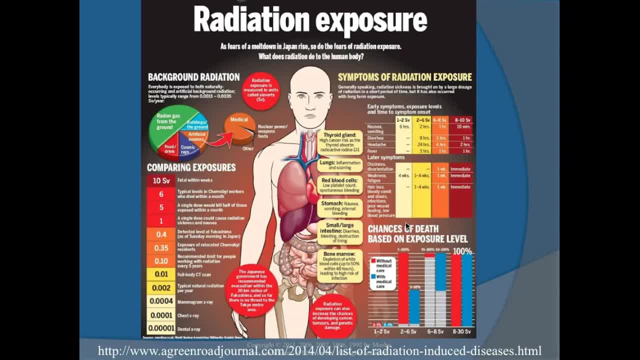 pretty good graph and it shows you our background here and then our medical little piece of pie there and you can see comparing exposure rates. so dental chest, mammo, natural per year CT. then we have the recommended limited exposure rates and then we have the recommended limited limits for people working in radiation exposures to Chernobyl. we had detective 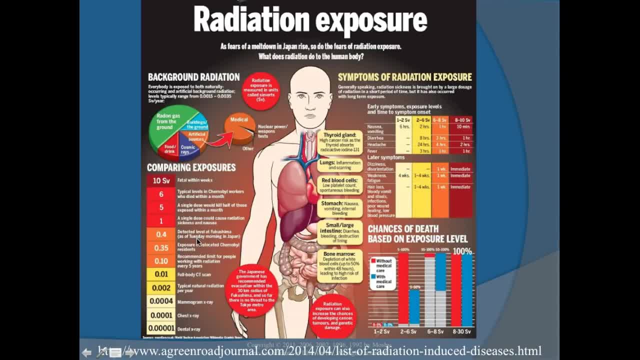 levels of Fukushima, which is very, very sad, and then a single dose could cause radiation sickness and nausea. so here, this is where we're starting to see some, some big effects, and we have: a single dose would kill half of those exposed within a month, and then we have the typical levels of 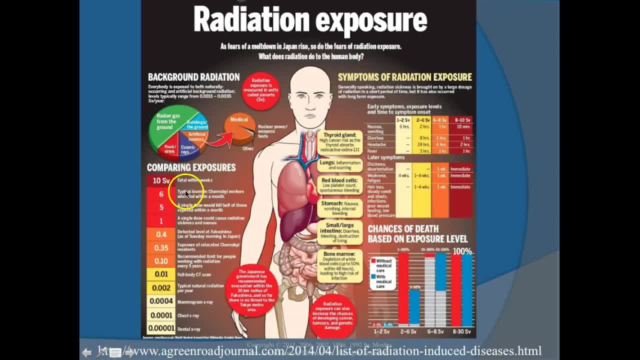 Chernobyl workers who died within a month- so right there- and then fatal within weeks, is 10 sieverts, yikes. so you can just take a look at this and you can see the different areas that the body will react to radiation and the levels at which you're gonna see changes within the body. okay, so protecting the patient. 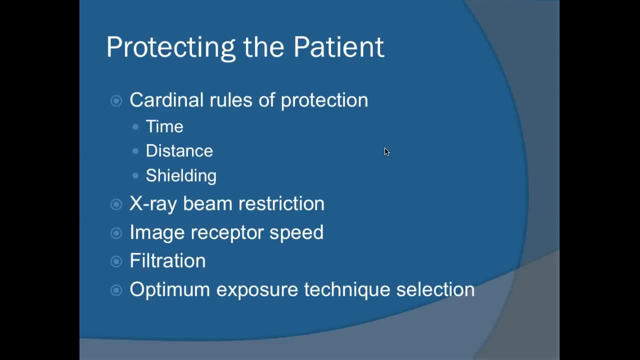 there's cardinal rules for protection. what are they? time, distance, shielding. you should know this. so we want to reduce the time, we want to increase the distance and we always want to wear shielding and protect the patient with lead. so x-ray beam restriction also. what does that mean? that's collimation image receptor speed. we want the fastest speed. 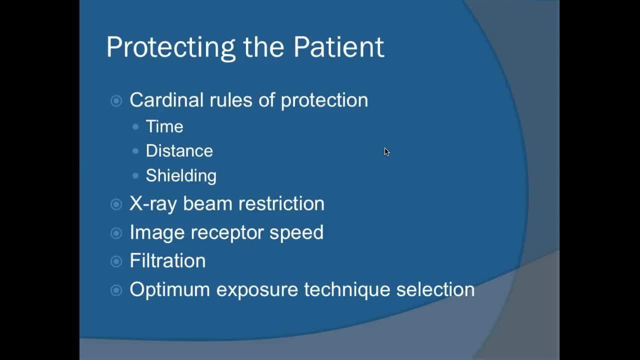 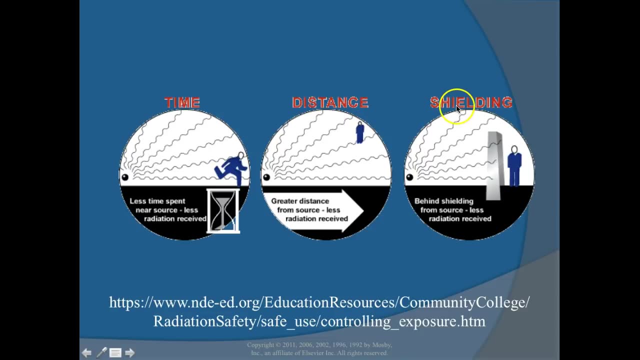 we want to use filtration to filter out the soft x-rays and we want to use the optimal exposure technique selection. so here you've got: your time, your distance and your shielding. so less time spent near the source, less radiation, and received greater distance is the less radiation received. that's based off the inverse square law and standing behind a 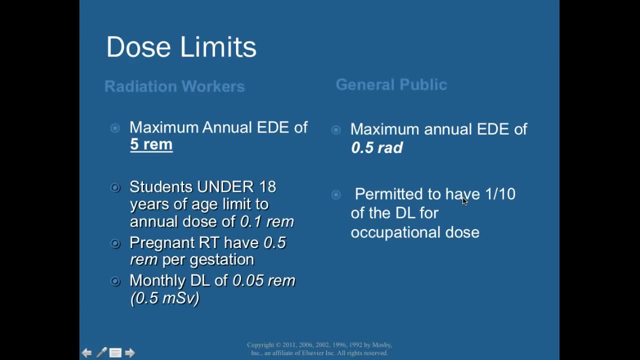 barrier will also reduce your radiation exposure. so dose limits, here we go. the annual ED is 5 rem. so students under 18 years of age limit the annual dose to 0.1. I've never had a student under 18, I can't imagine. but the pregnant worker is. 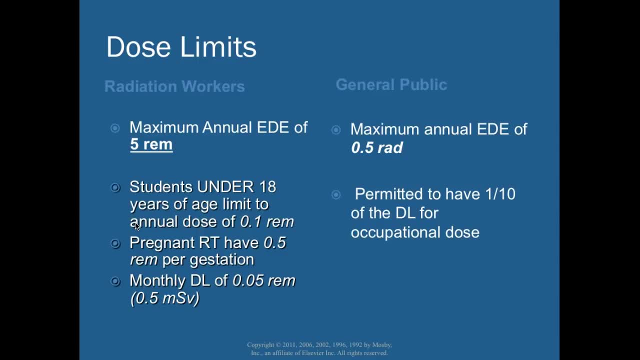 0.5. you have to know these, so pay attention. annual ED for radiation workers is 5 rem. students a are 0.1 rem, pregnant point 5 rem and then per gestation. so it's important to clarify that. so they're only allowed to receive. 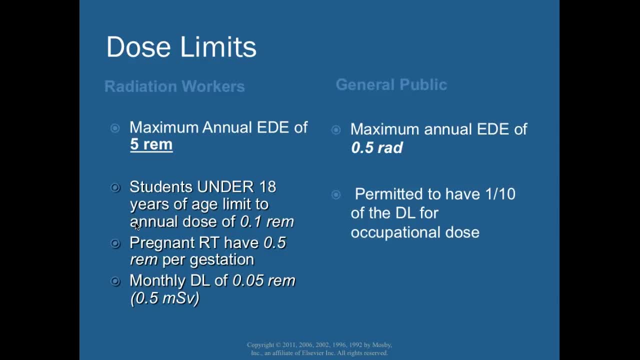 0.5 rem per gestation and that's they actually were led and clipped the radiation badge under the lead and then the monthly dose limit is 0.5 rem, limit of 0.05 rem or 0.5 millisieverts if you're looking at a monthly. so if you 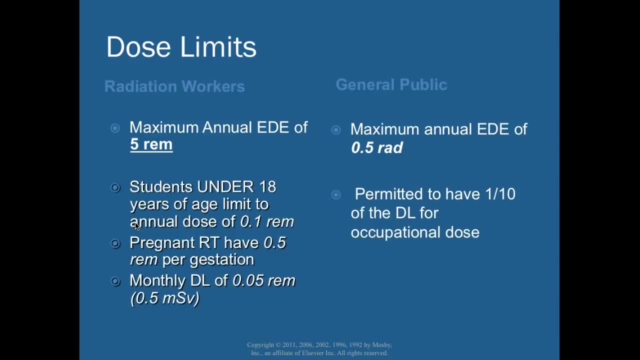 get zapped one month. I have to regulate that and make sure you don't exceed that amount for a month. okay, so for the general public, the EDEs: 0.5 rad, rad. do you notice how it changed from rem to rad? so rem is what we are looking at for. 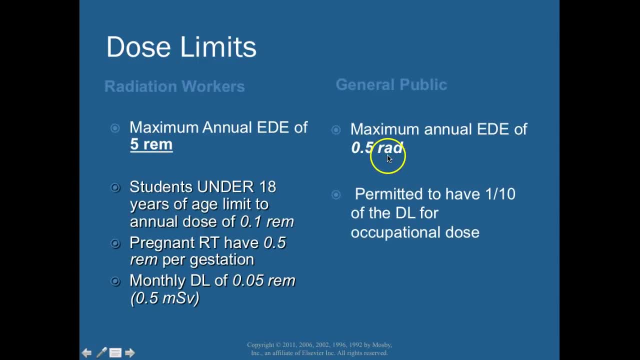 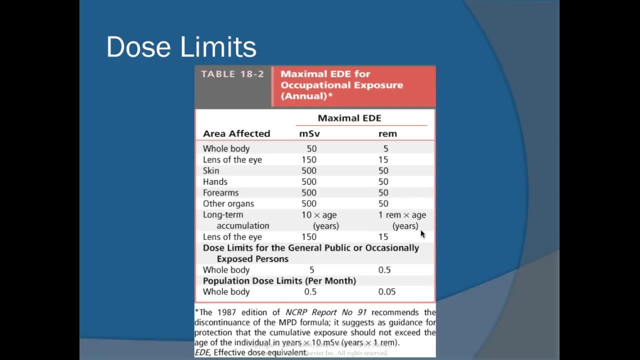 the worker and rad. why do we switch to rad radiation-absorbed dose, so this is absorbed. this is general public permitted to have one-tenth of the exposure as occupational workers. okay, so looking here as you can see the whole body versus all the way down the lens of the eyes sensitive. we have to be careful. 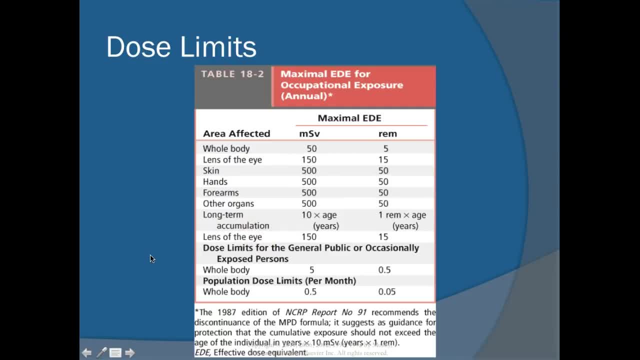 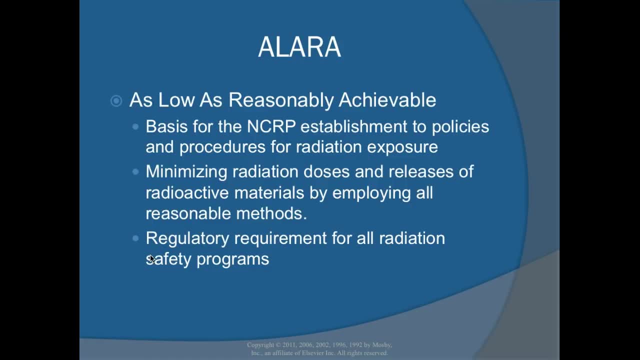 with the lens of the eye and just kind of gives you an idea of what we're, what we're looking at here. okay, Alara, so we've covered this before. I'm going to give you a little assignment on your Alara. so it's the basis for the NCRP establishment, two policies and 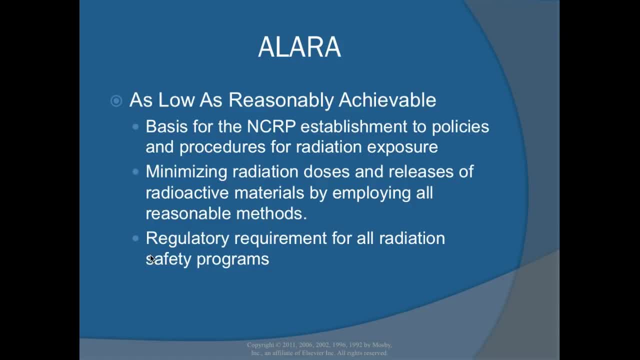 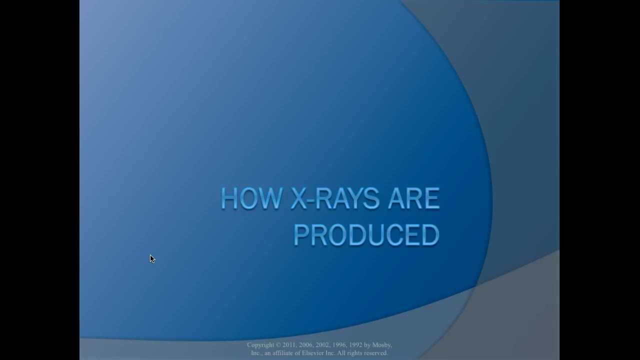 procedures for radiation exposure, so minimizing radiation dose, doses and releases of radioactive materials by employee. all reasonable methods, so regulatory requirements for all radiation safety programs. now let's get down to how x-rays are produced, and this is where we're going to go into you, not so much exactly what happens inside of the tube, but kind of what happens in. 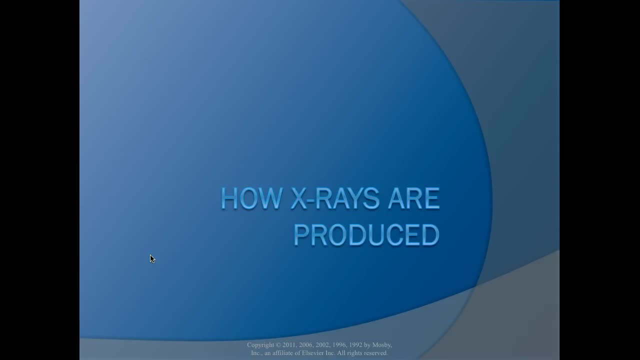 the tube general and then what happens within the body. so we're going to cover this, we're going to go deeper into this next semester, so we're just going to kind of introduce it for you. okay. conditions necessary for x-ray production: as we talked about over the summer: you have to have a source of. 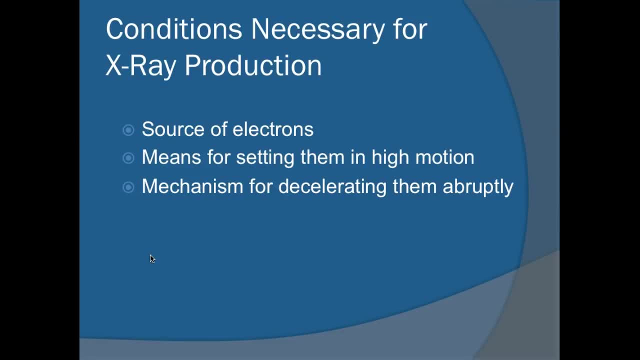 electrons, you have to means for setting them into high motion and you have to have a mechanism for decelerating them abruptly. so the source of electrons, remember it's the electrons are boiled off of the filament into an electronic cloud, means for putting them into high motion. we apply kVp in a potential difference so that 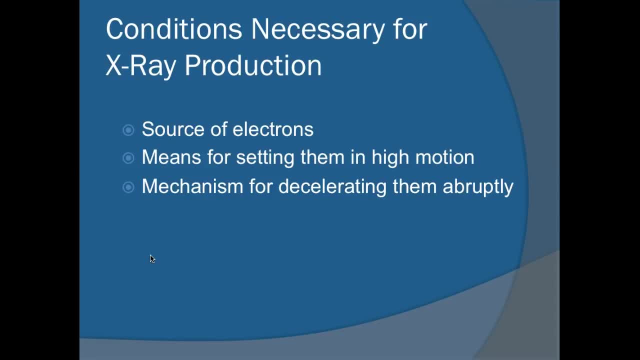 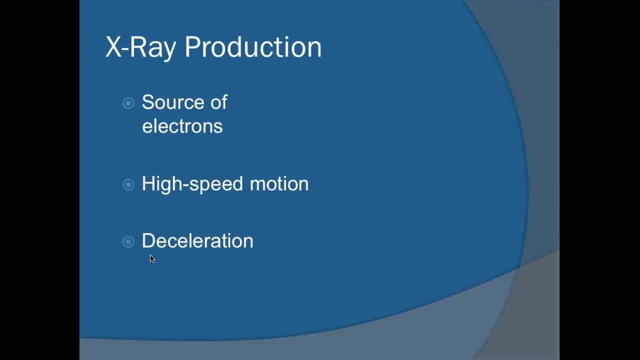 the electrons fly across to what the anode hits. the anode, that's the deceleration, so it stops them abruptly. that's how we get x-rays photons, all right. so the source of electrons we get from the filament, and the high speed motion is where we do the potential difference in. 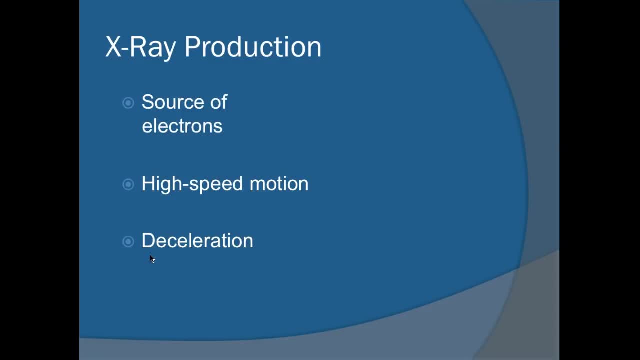 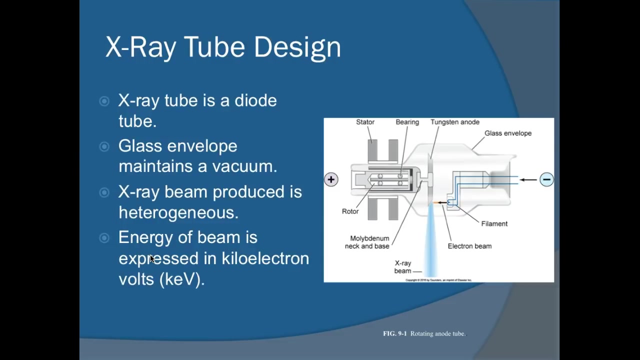 the kVp and then did: deceleration is on the anode when it hits the tungsten target, right, alright, oh, look, how fancy we are. alright, oh, my goodness, here we go. okay, tube design. x-ray tube is a diode tube, so there's a glass. 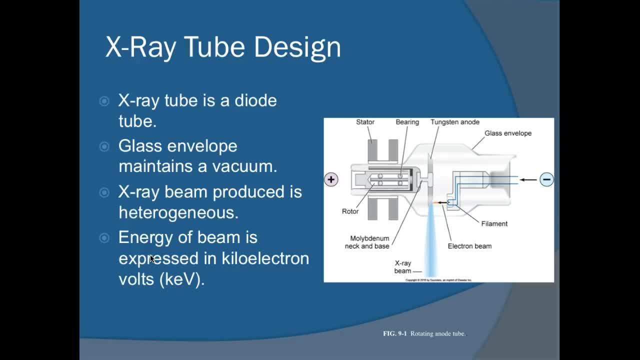 envelope that maintains the vacuum the x-ray beam is produced is heterogeneous. so what does that mean? it means that they're all coming off at different speeds, so they're not homogeneous, which means they'd all be the same. they're heterogeneous, so there's a kind of a bell-shaped curve. so we come- it'd be like this and you would- 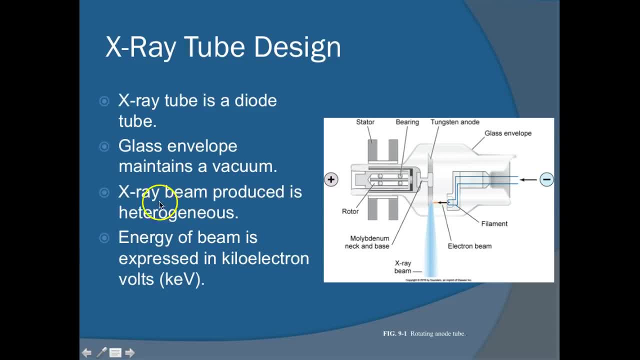 have, you know, 70 kVp here and zero here, and the average would be a lot less. so the energy of the beam is expressed in Kilo electron volts, so KeV. okay, so the energy of the beam is expressed in KeV. we're used to KVp kilovolts peak. this is 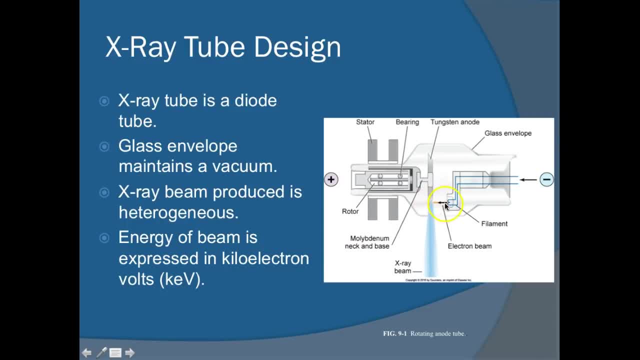 kilo electron volts. so here we're dealing with electrons, right? they're not photons yet. so kilo electron volts, so this is your electron beam, right here. so here's your filament, here's your anode and your tungsten target. you're looking at your electron beam and you're looking at your anode and you're. 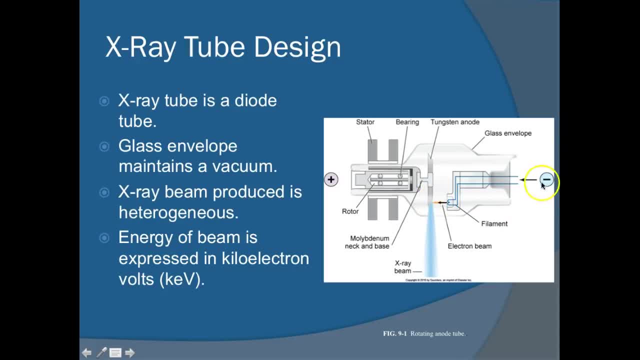 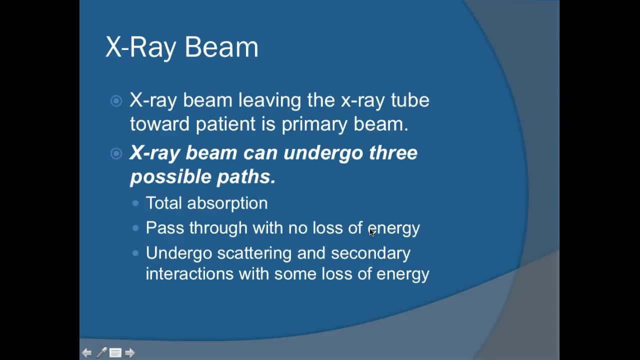 so they come across with the potential difference. so you have negative. negative to positive and that's how we we produce electrons. so the x-ray beam leaves the x-ray tube toward the patient is called the primary beam. so x-ray beam can undergo three possible paths: total absorption within the patient. it can. 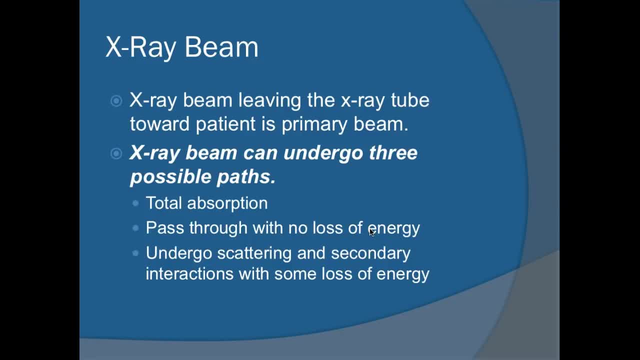 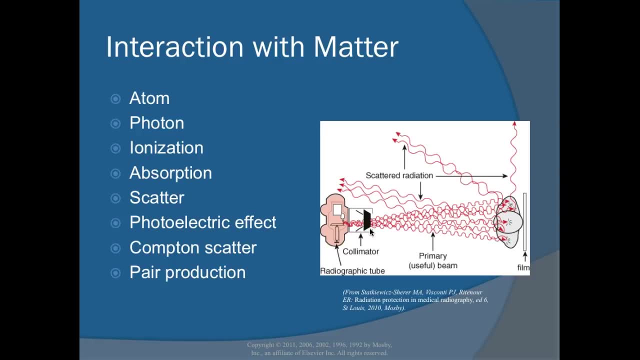 pass through the patient with no loss of energy, or it can undergo scattering or secondary interactions with some energy that is lost. so, looking here, it can interact with atoms, photons. there's ionization- that happens, there's absorption- that happens, scatter that happens. then we're going to 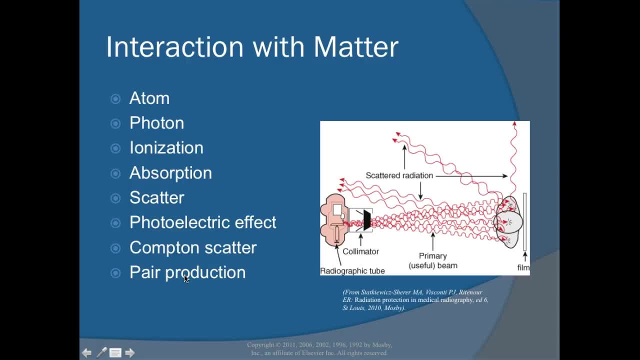 look at photoelectric effect, compton scatter and pair production and we're going to look at photo dissemination integration also. so key is to pretty much eliminate the zone which is the giant scale, and really Here we've got the x-ray tube, the anode, cathode anode and the electrons shoot across. 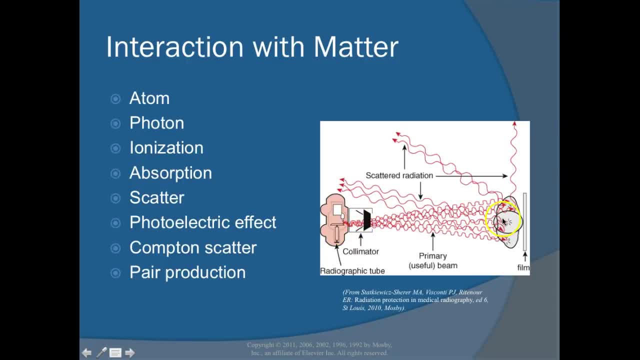 Now we have photons coming through and they're coming out. They're hitting the patient. They can be totally absorbed. so you can see here it's not exiting the patient, It can be scattered so they can come off in any direction. 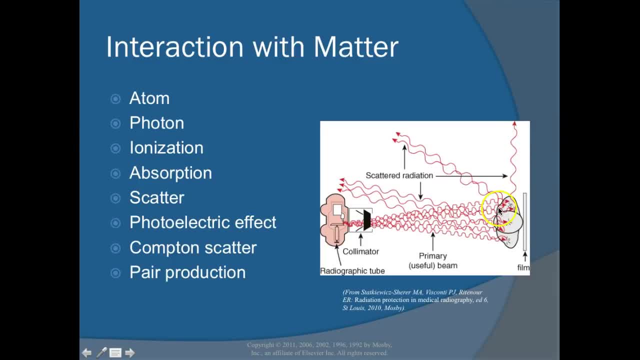 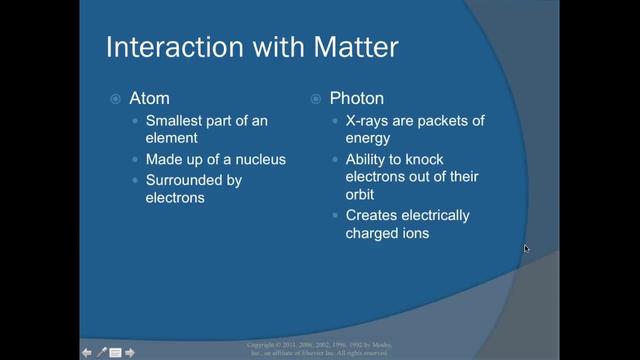 They can come straight back at you- It's called backscatter- or they can be off at any angle, or they can pass through and hit the IR. So basics here. Atom: smallest part of an element. It's made up of a nucleus surrounded by electrons. 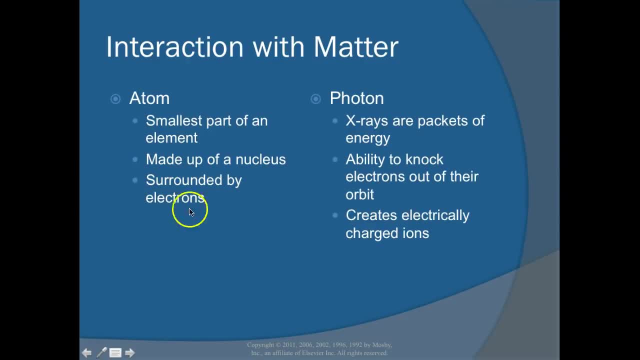 This is the key part: It's surrounded by electrons, okay, So keep that in mind. So a photon or x-rays are packets of energy. They're able to knock electrons out of their orbit and it creates electrically charged ions. 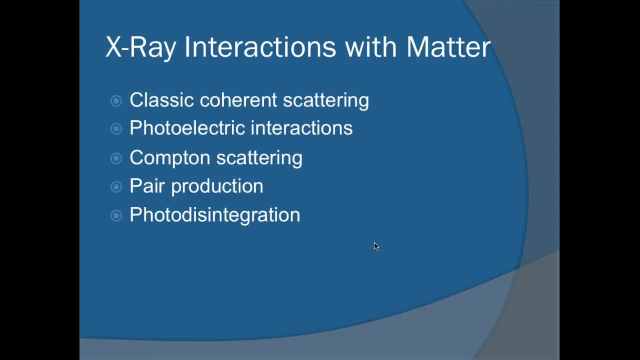 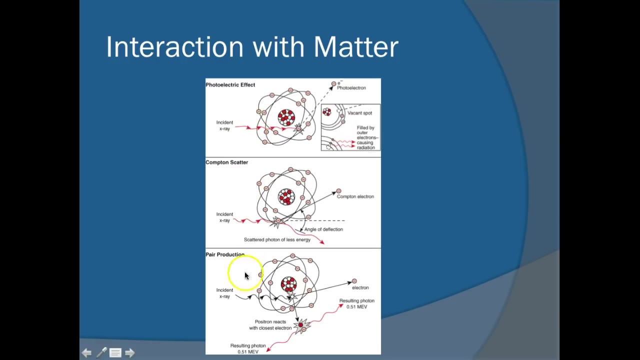 So There's different interactions that we have with matter. There's classic or coherent scattering, There's photoelectric interactions or absorption, There's Compton scattering pair, production and photodisintegration. So here's photoelectric Compton and pair. 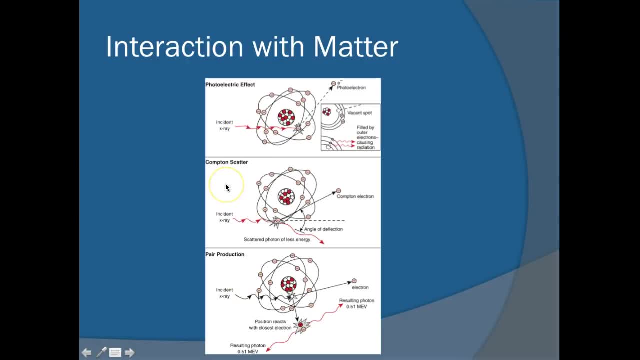 These two, photoelectric and Compton, are the two that we work with in diagnostic x-ray. Pair production happens in radiation therapy. Pair production and photodisintegration- The classic or coherent scattering- happens with mammography. So we're going to discuss that. 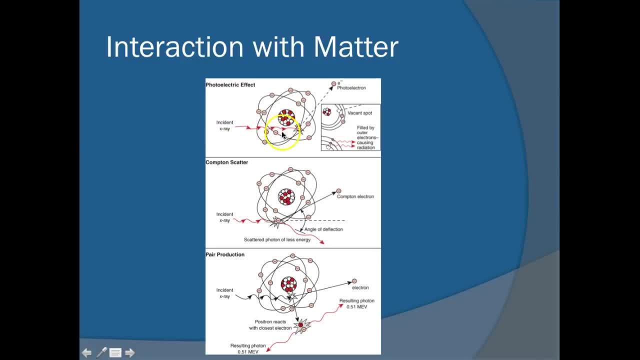 So here we have photoelectric effect coming in. Here's your incident: x-ray Comes in and knocks out a shell, and you have a photoelectron. You have Compton comes in, knocks out a shell here and you have a Compton electron. 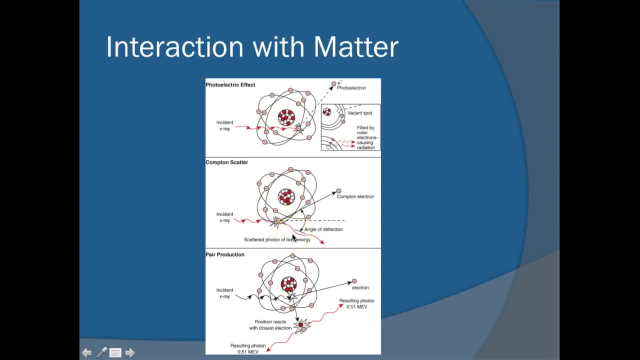 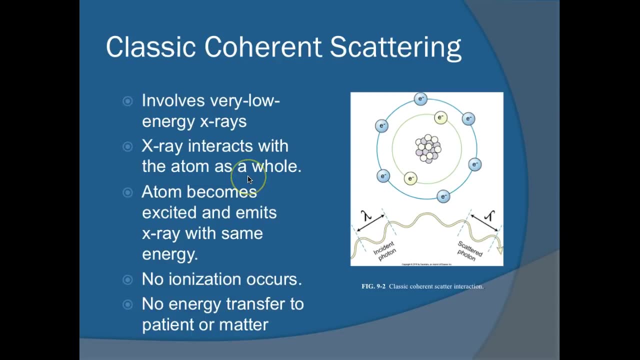 And then we look at this angle of deflection of the scatter. So let's start from the basics here. So classic or coherent scattering involves very low energy x-rays. X-rays interact with the atom as a whole. The atom becomes excited and emits an x-ray with the same energy. 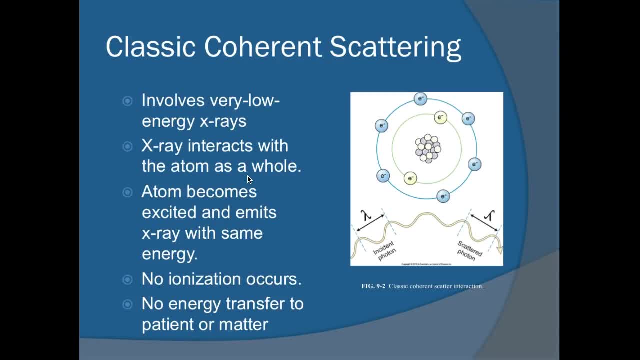 So no ionization occurs and no energy transfers. So this usually is in mammography, where we use a really really low kVp. We'll go anywhere from like 25 to 35 kVp and this is what happens. 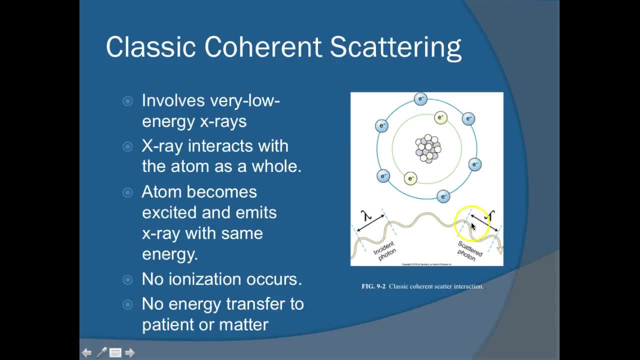 So it comes through and it you can see. the wavelength is the same. so the incident versus the scatter. So scatter is considered a scatter, photon is considered any photon that changes direction. So you have the incident coming in and you can see here. 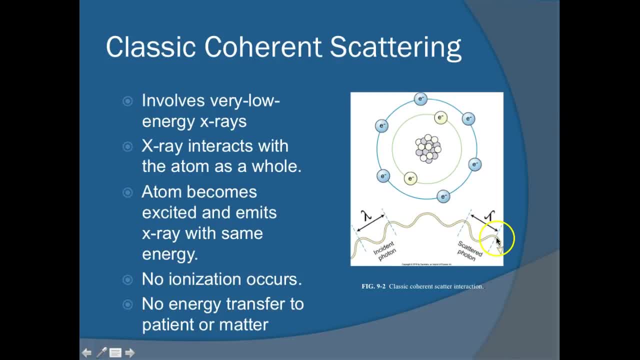 whoa lost it. So it's coming in and it changes, but we don't have an energy loss, It's the same. So it changes direction, makes this whole thing vibrate, okay, and it vibrates and it gives off a ray, okay. 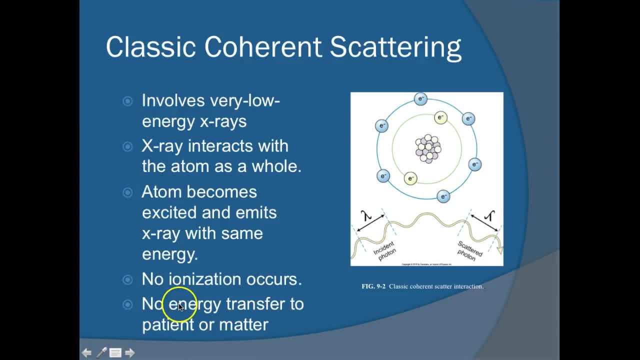 So just memorize this little chain of events here. So very low x-rays interacts with the atom as a whole, becomes excited and emits an x-ray with the same energy. No ionization occurs, no energy transfer to the patient or matter. okay. 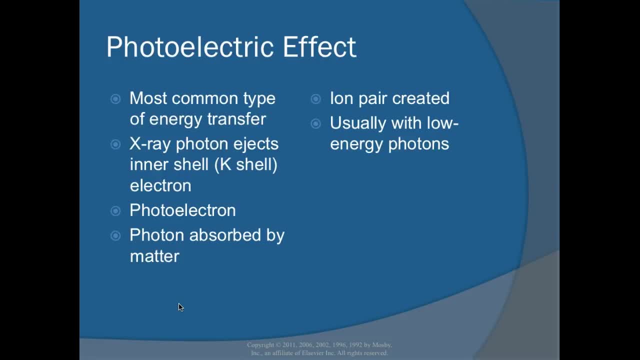 Photoelectric. So it's photoelectric effect or photoelectric absorption. You're going to see it both ways. I don't want you thrown off. So it's the most common type of energy transfer. X-ray photons eject an inner shell, k-shell. well, it's k or l. 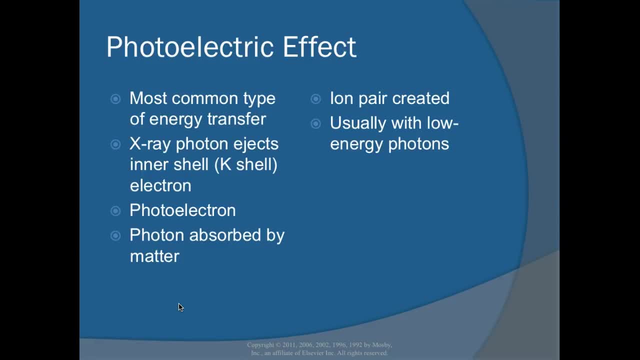 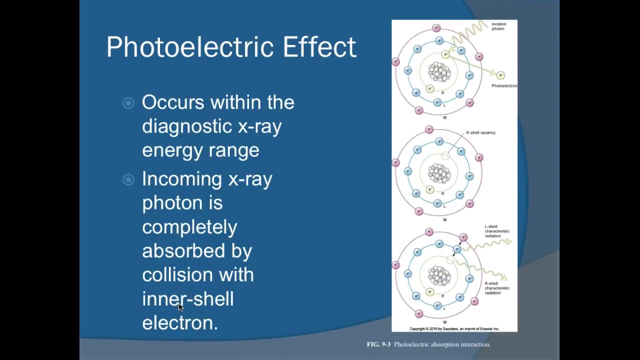 shell electron, You get a photoelectron and the photon absorbed by the matter, So an ion pair is created and usually low energy photons. So this is lower energy than Compton but higher than your classic, Alright. so 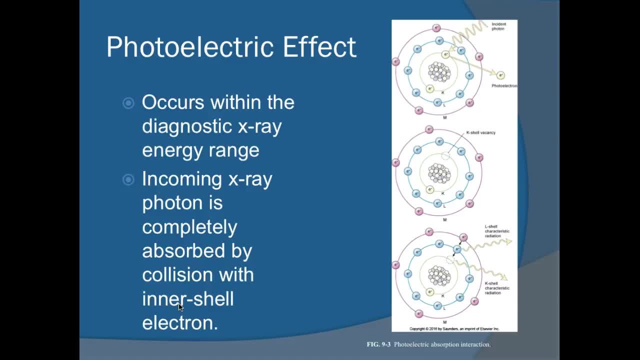 occurs within the diagnostic x-ray range. So the incoming x-ray photon is completely absorbed by the collision with the inner shell electron. So it's usually the k or l shell that it's hitting and you can see the incident comes in and knocks it out and it's called a photoelectron when it knocks it out. 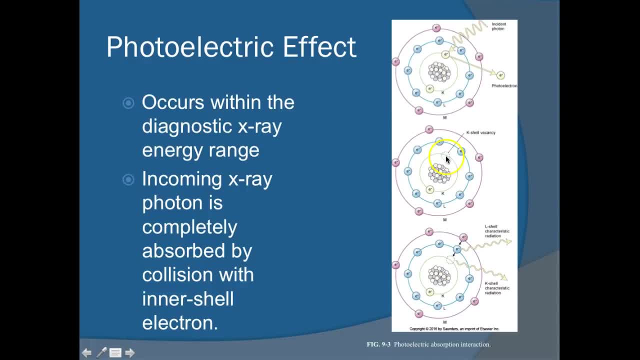 There's a vacancy here, which makes this very unstable. So you have to have a shell, a higher number shell drop in to the inner shell and when it drops in you get a characteristic photon that comes off, So it gives off energy when it drops down into the lower shell. 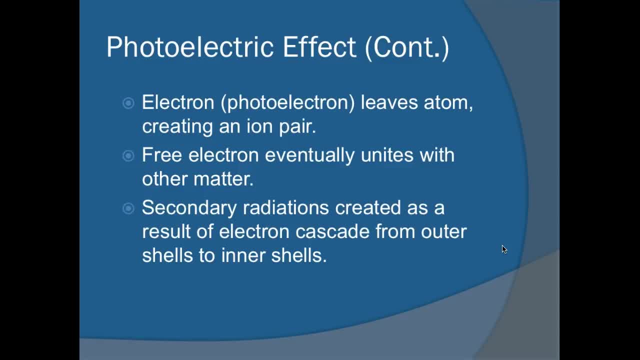 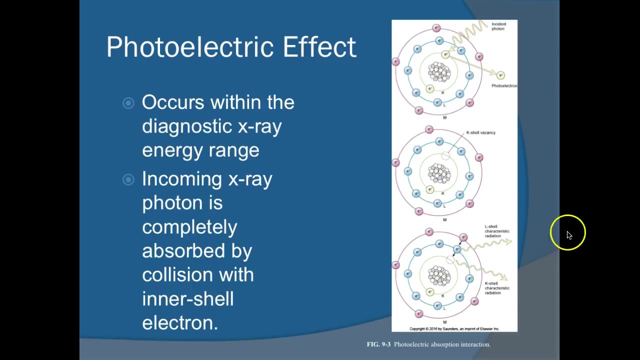 So the photoelectron leaves the atom, creating an ion pair. The free electron eventually unites with other matter and is absorbed completely. The secondary radiation created as a result of the electron cascade from the outer inner shell, so this is called. 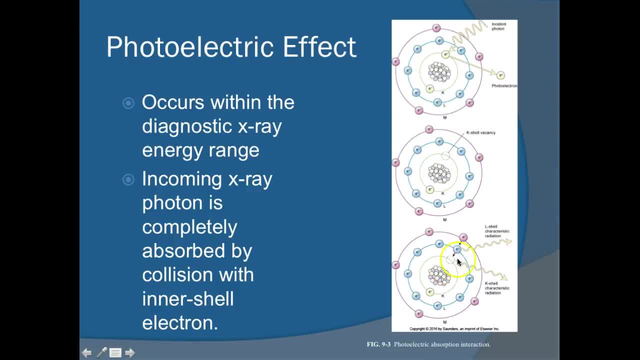 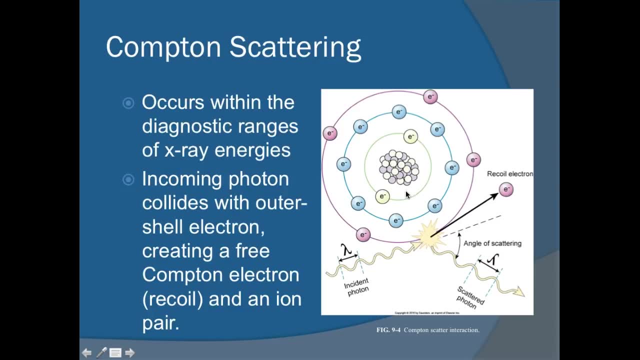 cascade, characteristic cascade. So as each one drops down it gives off this characteristic cascade of radiation. Alright, So Compton alright occurs with within diagnostic x-ray energies. So the incoming photon collides with an outer shell electron, creating a free Compton. 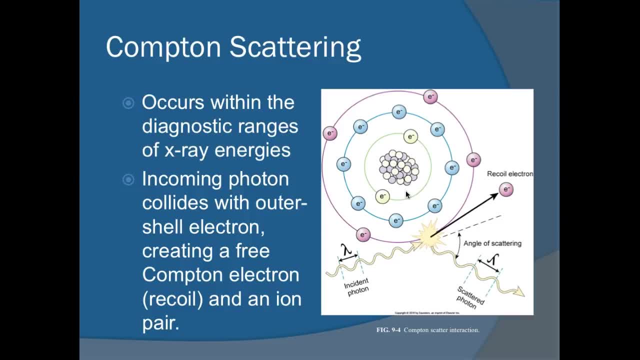 electron, or what we call a recoil and an ion pair, So it comes in. so photoelectric hits an inner shell, Compton hits an outer shell, So it comes in. the incident: photon hits one of the electrons, knocks it out, and this is called the recoil electron. And then 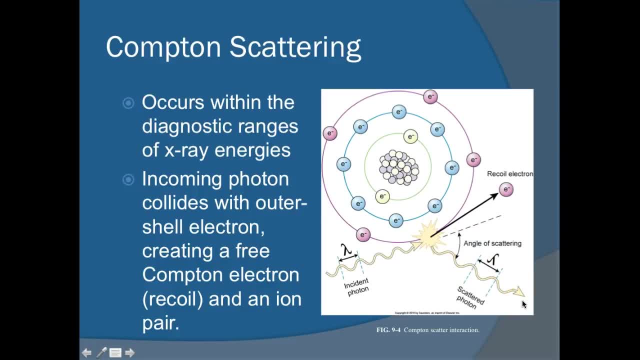 you have a wave coming off here, So this is called the scattered photon. So you have a recoil electron and a scattered photon, giving you an ion pair. Okay, So the angle of deflection: we're going to talk about that more in. 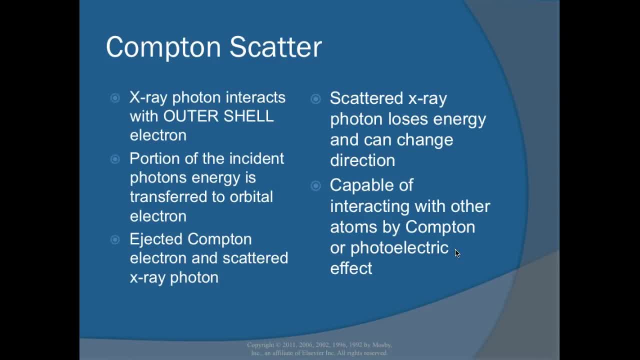 next semester. So with Compton scatter the x-ray photon interacts with the outer shell electron Portion of the incident. photon energy is transferred to the orbital electron and ejected Compton electron and scattered. ejected Compton electron and scattered x-ray photon. So you get both. 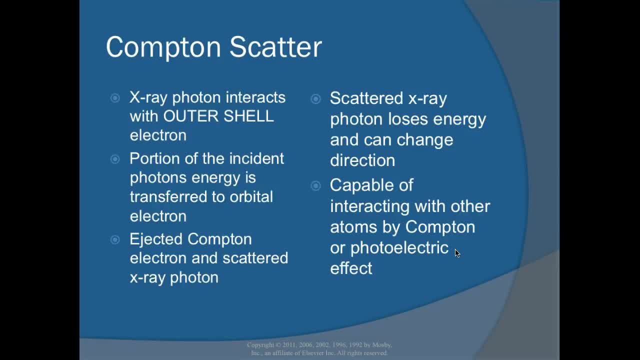 The scattered x-ray photon loses energy and can change direction. It's capable of interacting with other atoms by Compton or photoelectric effect. So, depending on the energy, it can do either another Compton interaction or it can be absorbed in photoelectric effect. 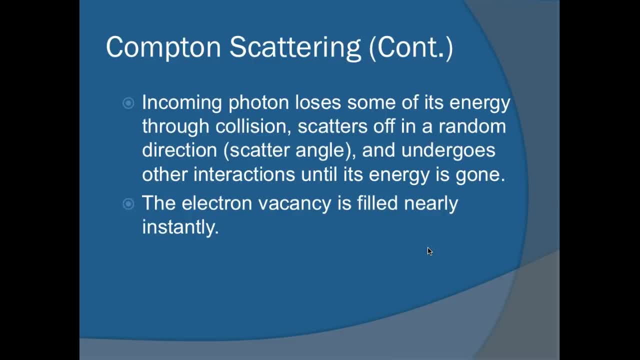 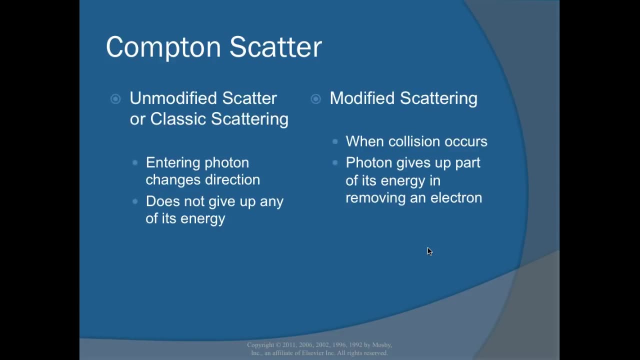 So the incoming photon loses some of its energy through the collision, scatters off in a random direction- So you have this angle- and undergoes other interactions until the energy is gone. So the electron vacancy is filled nearly instantly. So we have 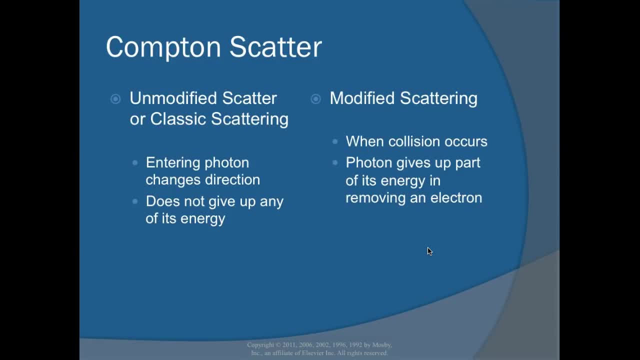 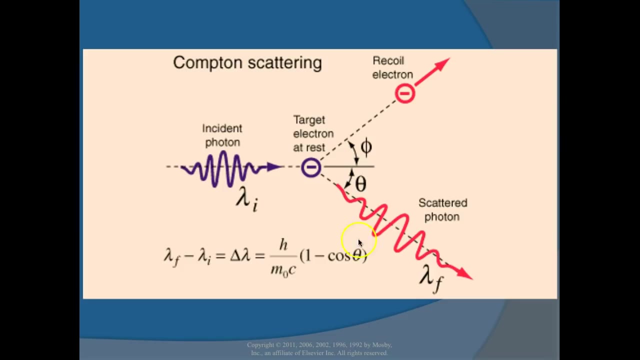 unmodified scatter or classic scattering. So the entering photon changes direction, does not give up any energy and you have the modified scattering is when the collision occurs. The photon gives off parts of its energy in the removal of the electron. So 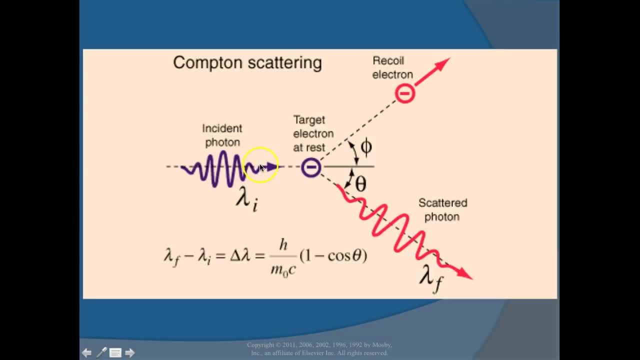 Compton incident: photon coming in around and it hits right the electron at rest. You have your recoil electron and you have your scattered photon. We can find the cosine of these angles, but we're not going to do it now, We'll do it later. 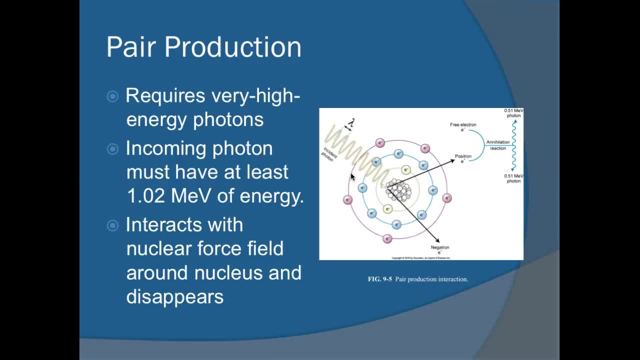 Para production. So now we are out of working with diagnostic x-ray, Now we're going into radiation therapy. So para production is higher energy photons. Incoming photon must be at least 1.02 MeV of energy. Interacts with the nuclear field around the nucleus and so you can see, here it comes in and 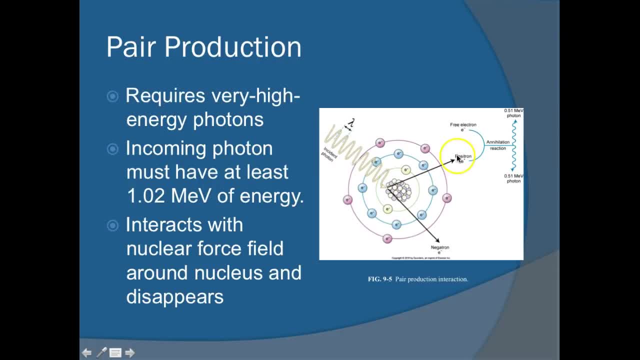 it hits the nucleus and it gives you a positive electron and a negative electron. So with a positive electron also has a free negative electron, You have annihilation, where it explodes again And you have .051 MeV photon and 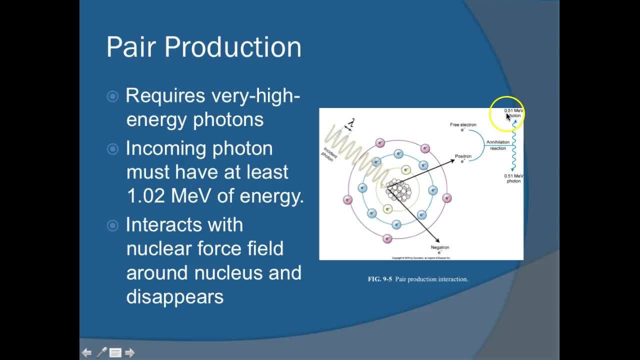 0.51 MeV photons. So when it splits you get this annihilation. so that's big, you got to remember annihilation. and then it splits off into two different photons, one at 0.51 MeVs. 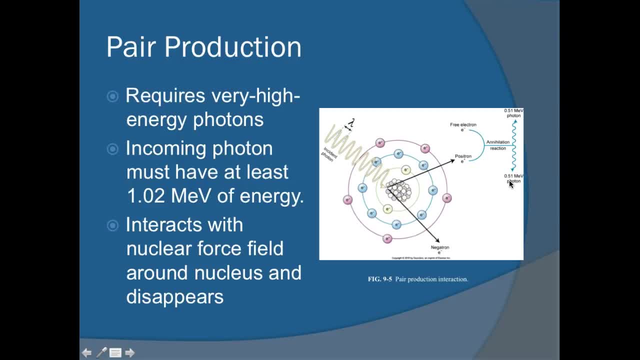 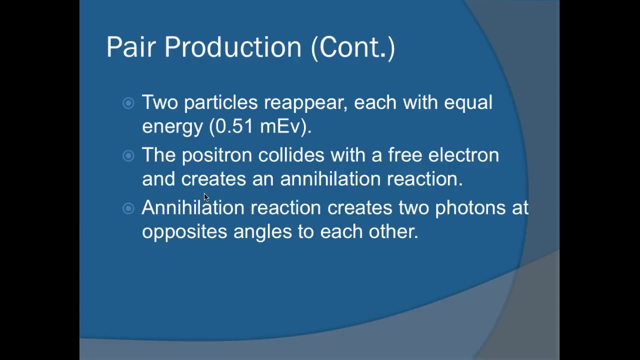 1 MeV and 1 at 0.51 MeV. okay, so the two together total 1.02 MeV of energy. okay, so more on pair production. we have two particles reappear, each with equal energy: 0.51 MeV. the positron collides with the free electron and 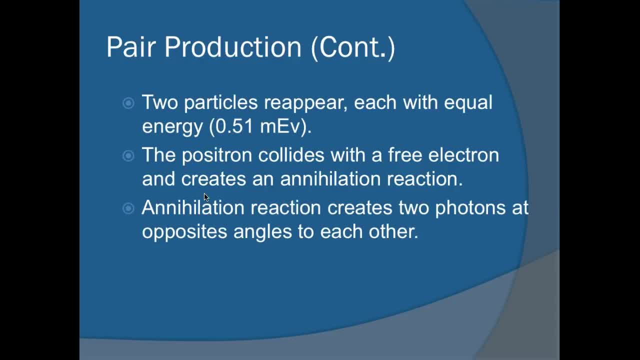 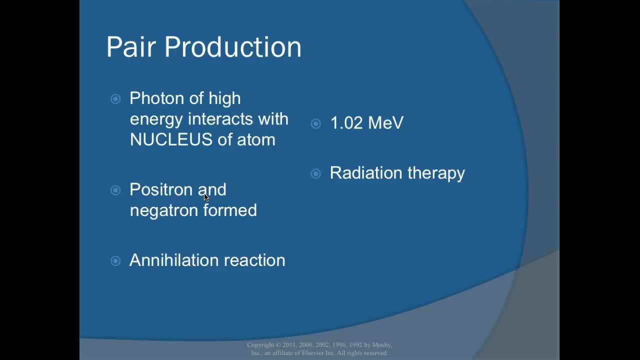 creates annihilation. annihilation reaction creates two photons at opposite angles from each other. so photons of high energy interact with the nucleus, so that's important. it interacts with the nucleus where in diagnostic x-ray we interact with the electrons right. so the nucleus is radiation therapy and that's. 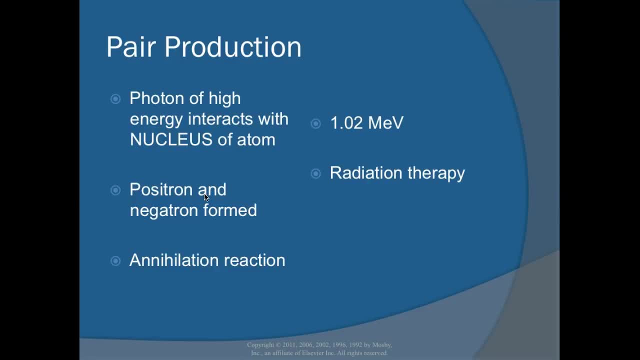 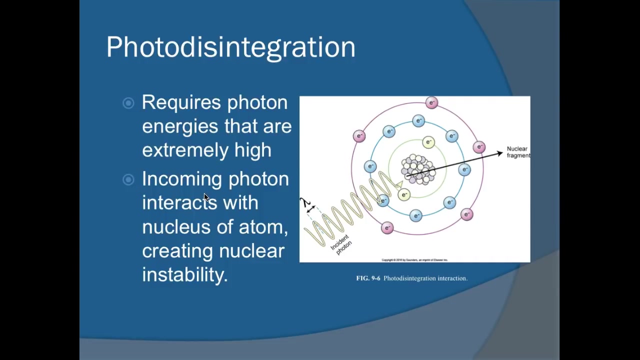 pair production and photodisintegration. so nucleus positron and a negatron are formed. annihilation reaction: you have the 1.02 MeV and you it's usually within- well, it's always within- radiation therapy. photodisintegration requires photon energies that are extremely high. 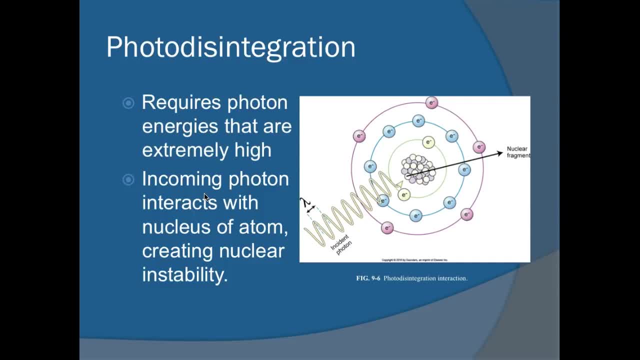 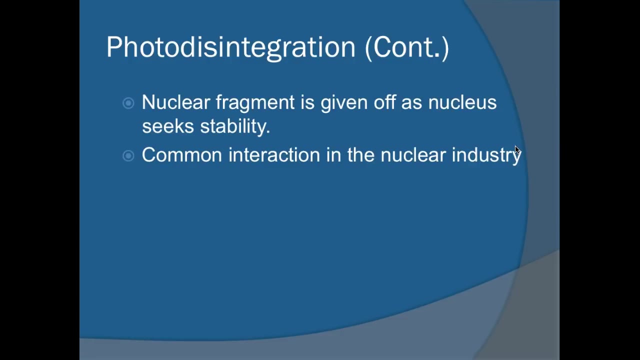 incoming photon interacts with the nucleus. there it is again of an atom, creating a nuclear instability. so comes in and then you get a nuclear fragment out. so that's really high. nuclear fragment is given off as a nucleus seeks stability, common interaction in the nuclear industry. so there you go, so by. 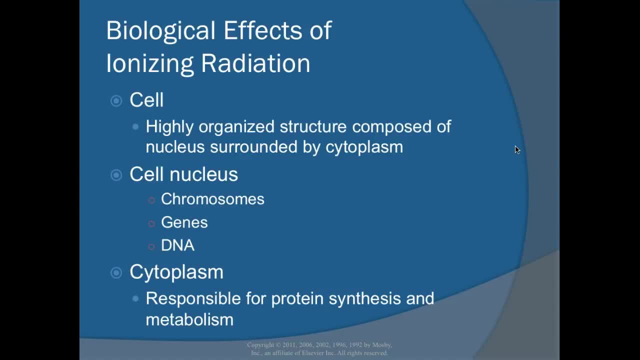 biological effects of radiation. so cells, highly organized structures composed of nucleus surrounding the cytoplasm, and then we have a cell nucleus, we have the chromosome, the genes and the DNA. any kind of hit in the nucleus is not good. the cytoplasm is responsible for protein synthesis and metabolism. so here's a review of the cell also, if you. forgot and biological effects of ionizing radiation. we have germ cells responsible for skin works in adiabatic preparation. that's my cliche. biological effects of ionizing radiation. we have germ cells responsible forünk biological effects of ionizing radiation. we have germ cells responsible for. 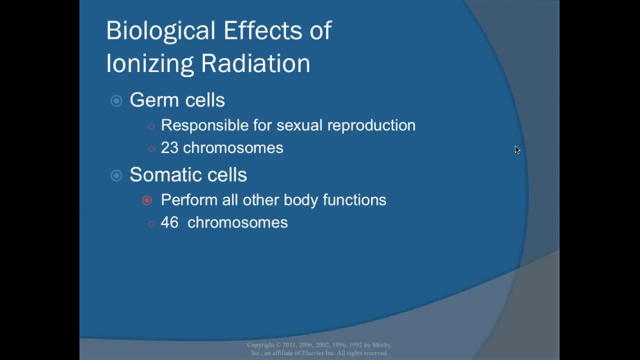 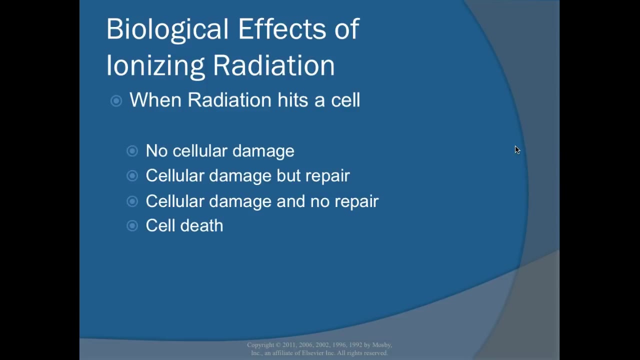 Picasso from Хот Uz Nat проект I MirafВ. sexual reproduction, so 23 chromosomes, and somatic cells perform all other body functions, so 46 chromosomes. and when a when radiation hits a cell, there's things that can happen, no cellular damage at all, which is great cellular. 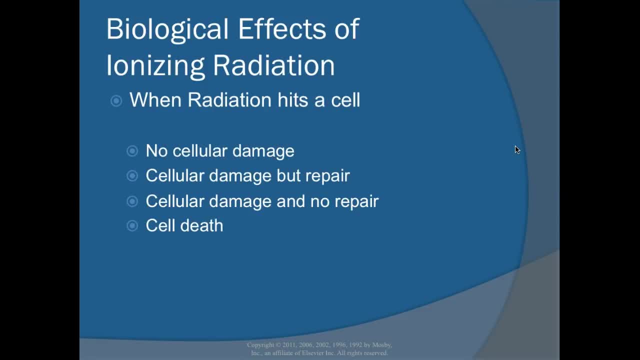 cellular damage but it can repair okay. so it's hit, it's damage, it's limping, but it can repair itself. then there's cellular damage with no repair, so the cell is either going to die or reproduce improperly and then there's cell death. so we are concerned here with cellular damage and no repair and cell 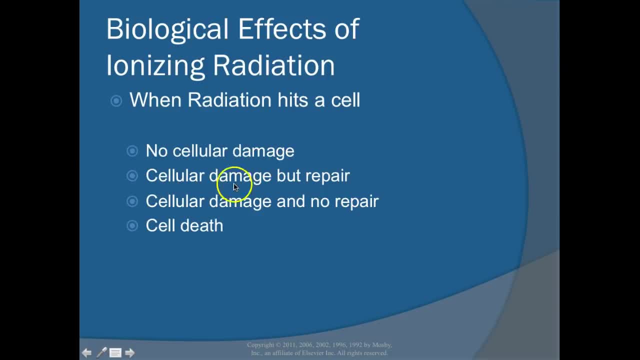 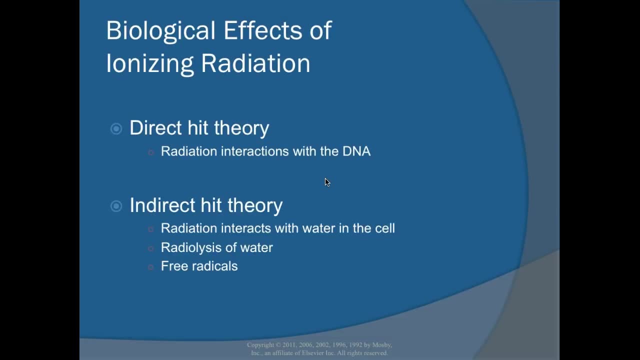 death. so no cellular damage, Yippee cellular damage, but repair. that's what we look for. we want the cells to be able to repair themselves. so we talked about the direct and indirect, so once again, review it. the direct hit is interactions with the DNA and the cell. so we talked about the direct and indirect, so once again, review it. the direct hit is interactions with the DNA and. 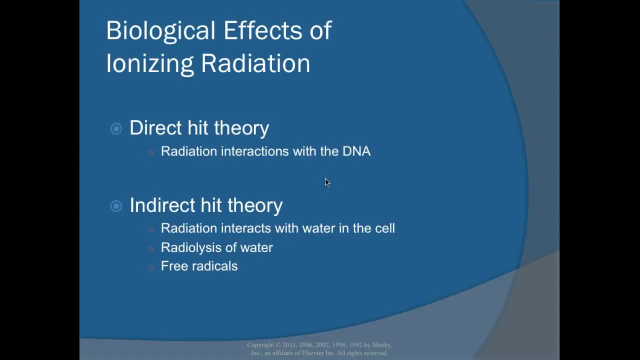 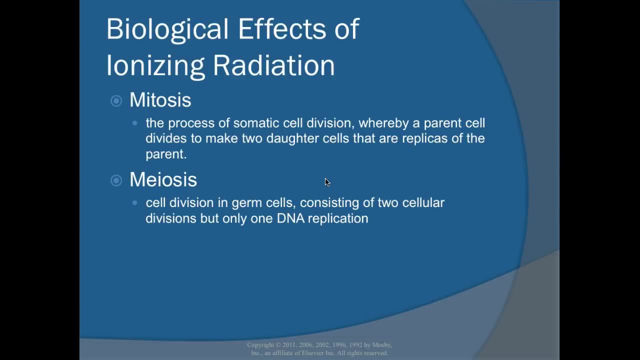 damage to the DNA and this is where the cancer comes from. indirect interacts with the water in the cell. there's radiolysis and free radicals. so mitosis, the process of somatic cell division, whereby a parent cell divides to make two daughter cells that are replicas of the parent. so with meiosis, cell division and germ. 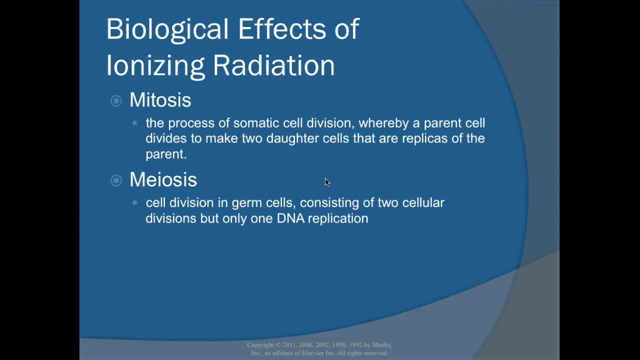 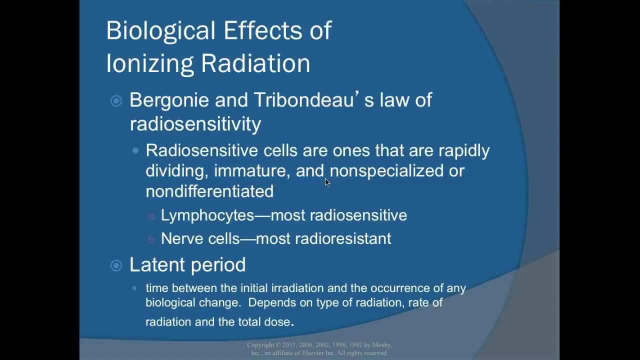 cells consisting of two cellular divisions but only one DNA reproduction, is합장 jakob's cell division. it's one cellular division, so the initial radiations of the DNA. so we can then take our cell and we can look at the different cell types and the same difference. alright, there's a burgundy's. 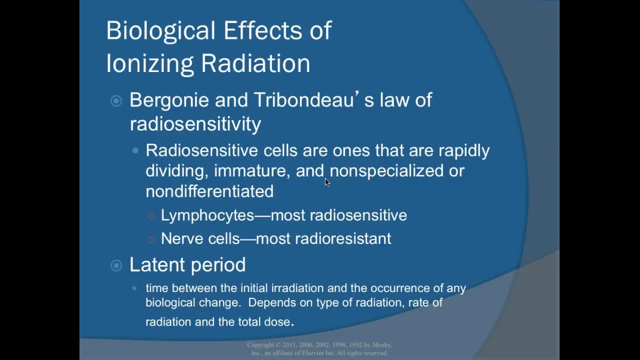 in to Bordeaux law of radio sensitivity. so radio sensitive cells are ones that are rapidly dividing, immature or non-specialized, or non differentiated. so lymphocytes are the most radio sensitive, where nerve cells are the most radio-resistant. so the latent period, what is late in period, is the time between: 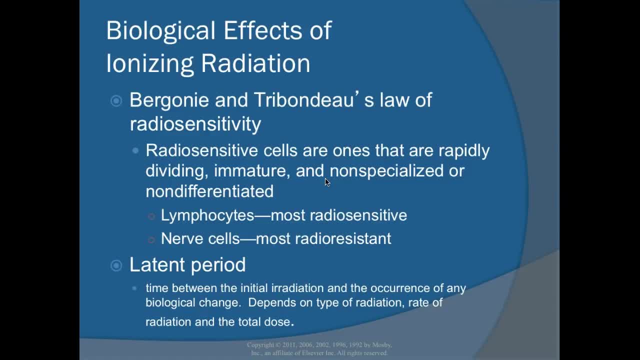 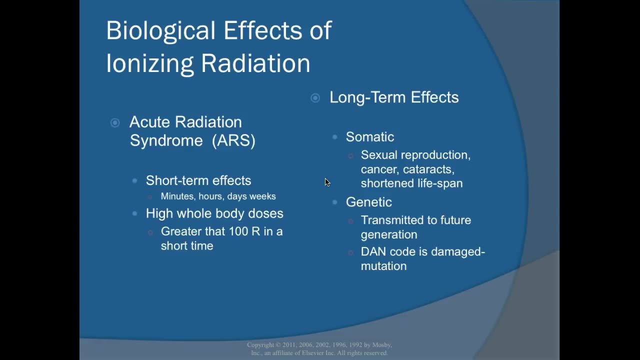 on the type of radiation and the rate of the radiation, along with the total dose. so if you're exposed at Fukushima, it depends on the amount of radiation that you received, on how long your latent period is all right. so with acute radiation syndrome- we're going to cover this again- short-term effects there's. 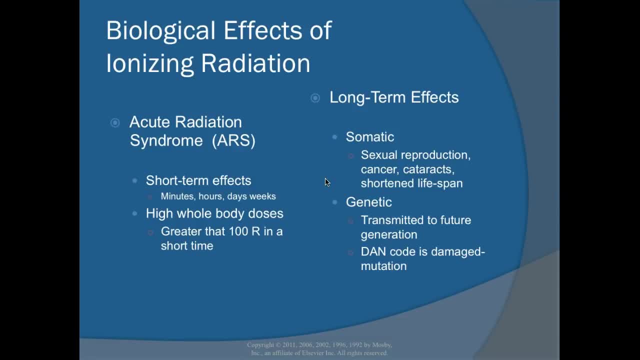 minutes, hours or days, weeks high. whole body doses are greater than a hundred, are in a short period of time, yikes long-term effects. they're somatic, so sexual reproduction, cancer, cataract shortens the lifespan. with genetic it's transmitted to future generations, so the Dan code is damaged. I think that's. 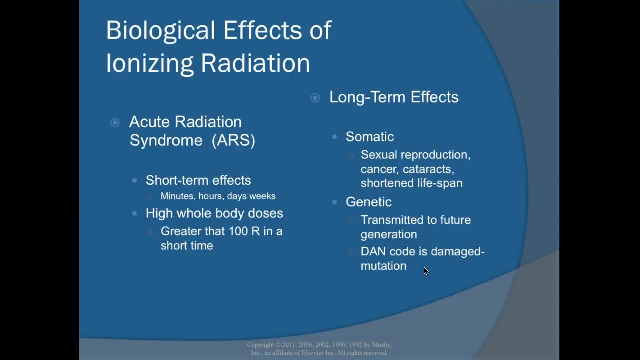 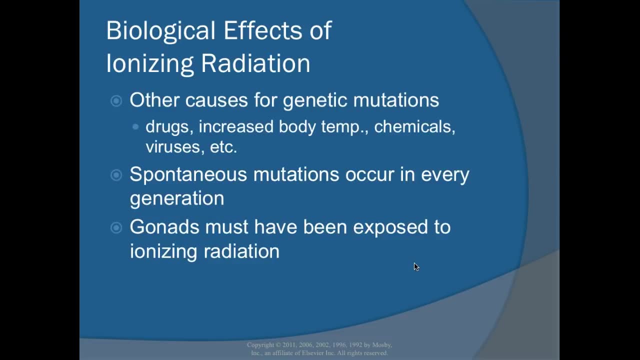 supposed to be DNA. that's interesting that they screwed that up. I didn't even catch it till just now. the DNA is damaged okay, so it's going to reproduce in properly. so other causes of genetic mutations- drugs, increase in body temperature, chemicals, viruses- spontaneous mutations occur in every generation. so we can't necessarily say 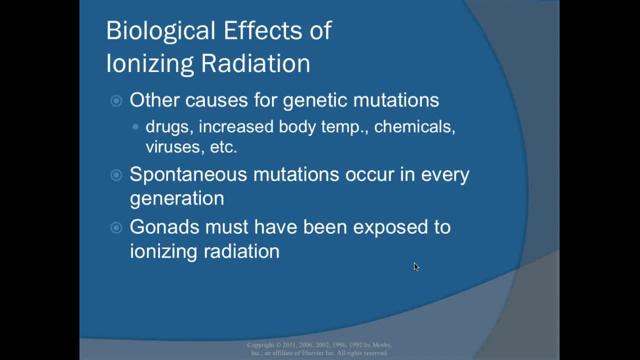 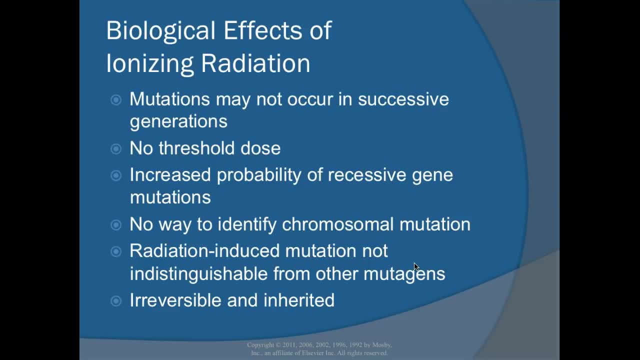 that mutations are from radiation. it's hard to prove. gonads must be exposed to an ionizing radiation to have that happen. all right, mutations may occur in successive generations, so there's no threshold dose. we talked about that increased probability of recessive gene mutations and no way to identify. identify. 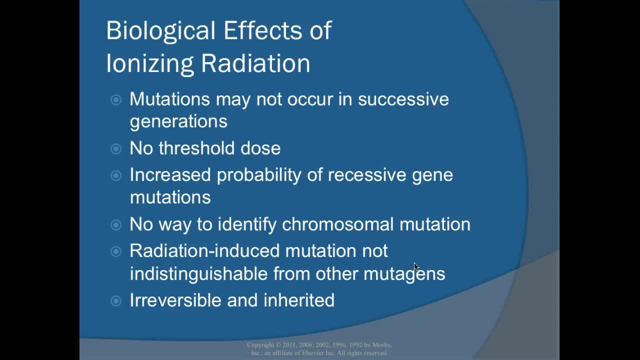 chromosomal mutations, radiation induced mutations not indistinguishable from other mutations. so that's where the hard part is. it's like: is that from the high dose of radiation that they received, or is this just a spontaneous mutation within that person's DNA? so the radiation exposures are irreversible and 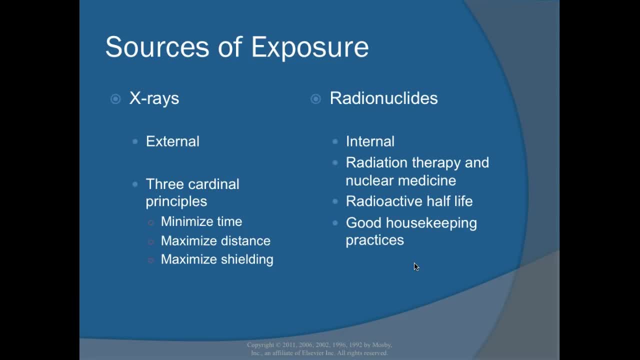 can be inherited. so sources of exposure, we have x-rays, so there's external and there's three cardinal principles, we talked about that already. so there's minimize time, maximize distance, maximize shielding. and with radial nuclei there's: they're more internal, so inside the body, so radiation therapy and nuclear medicine, radioactive. 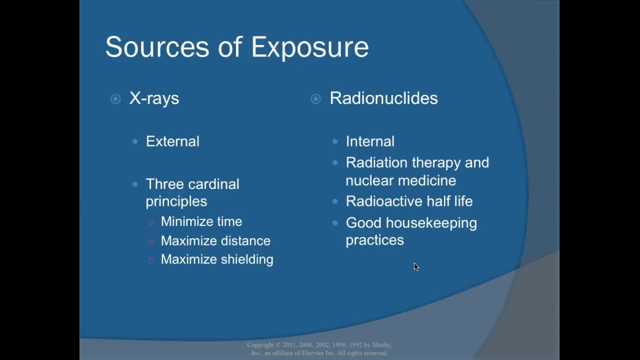 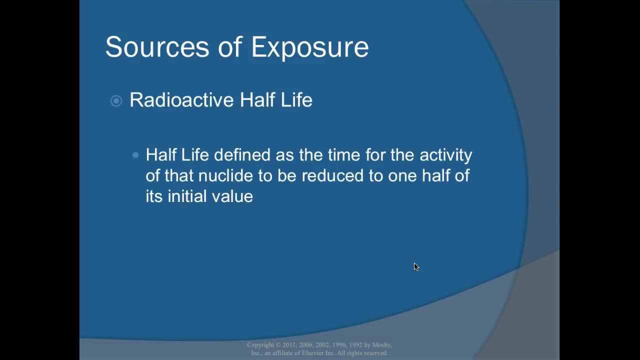 half-life when you look at that, and good housekeeping processes, alright. radioactive half-life- what is that? so the half-life is defined as the time for the activity of the nuclei to be reduced to one half of its initial value. so radioactive half-life, how do we get? 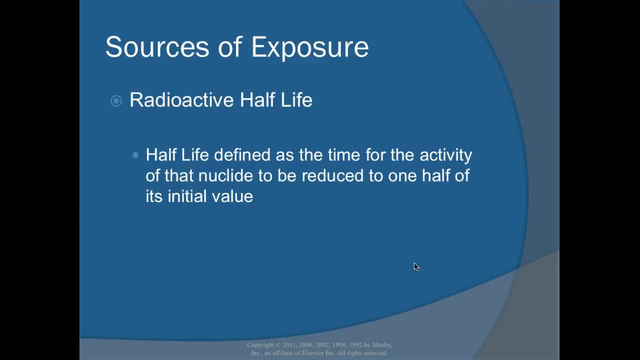 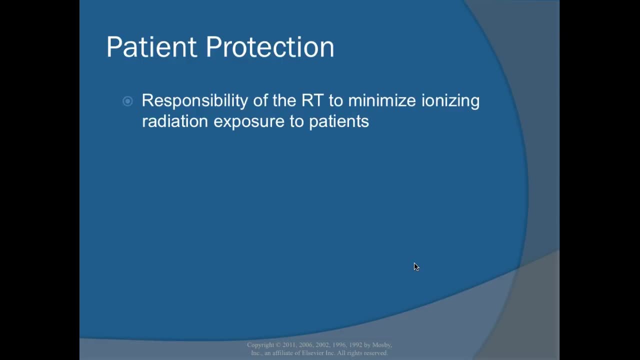 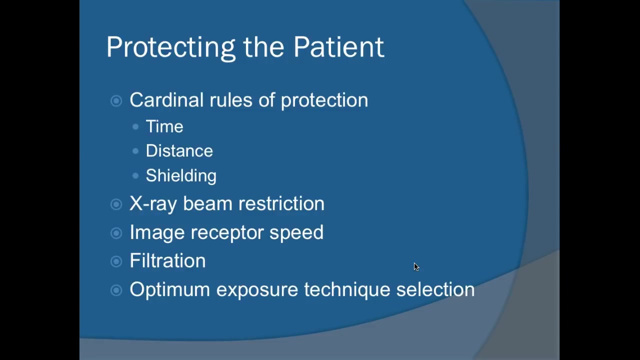 the radioactivity down to half. so that's considered the half-life. so patient protections responsible of the RT. so you need to make sure that the patient is protected and there's three cardinal rules. you want to reduce the time the patient's being exposed. you want to increase the 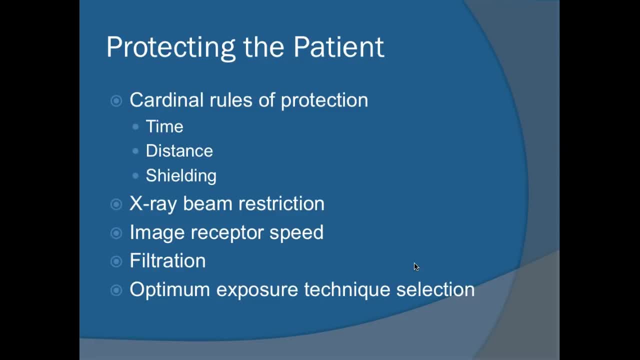 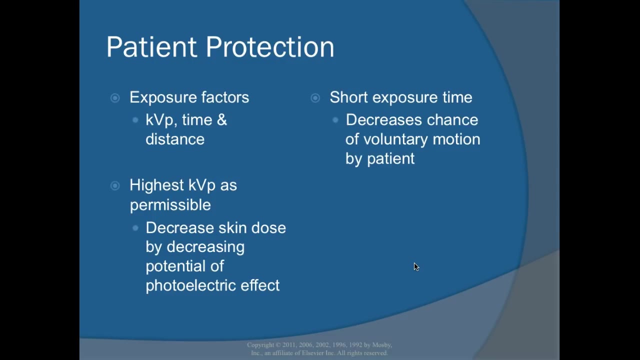 distance that you can for the patient. shield them when you can. you want to collimate and you need to use the fastest image receptor speed. you need to use the basic filtration to filter out the lower energy photons and pick the proper technique. so when we talk about exposure factors, we have the KVP time. 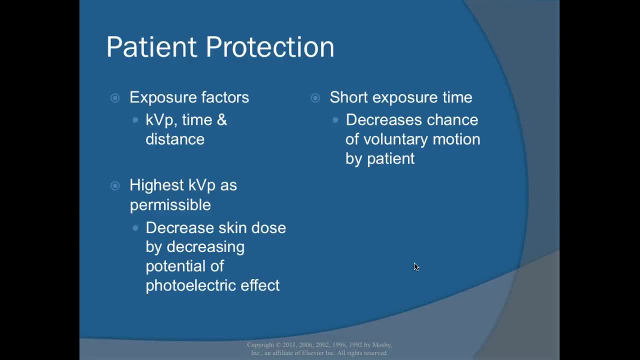 and distance. so you want to use the highest KVP that you can so that you're using Compton and hopefully the there's less absorption into the body. so you want to use high kVp to decrease the skin dose by decreasing the potential of photoelectric effect or absorption. short exposure times decreases the chances of 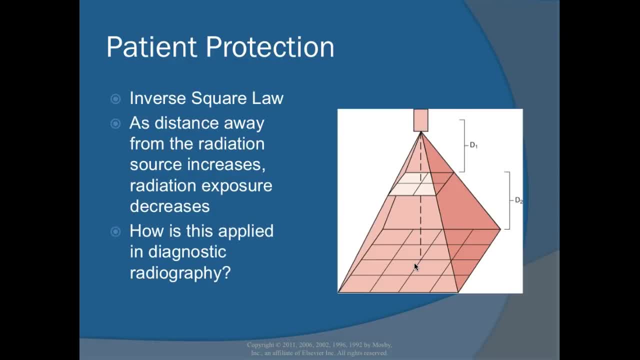 motion from the patient, so you don't have a repeat. so the inverse square law: as the distance away from the radiation source increases, the radiation exposure decreases. so here, as you can see, if you have a 10 by 12 here or 10 by 10, you 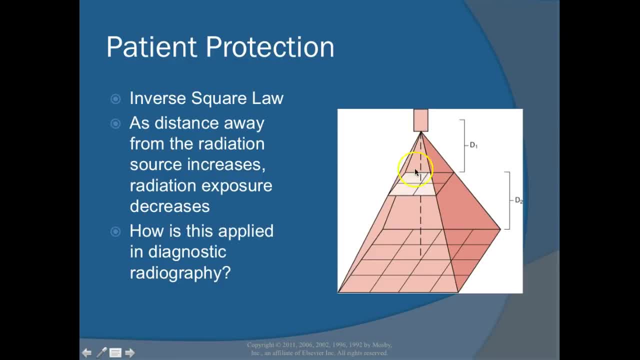 have your radiation source, you have all the photons hitting on this small piece. if you still had just the small piece, you can see there would be less photons hitting because they're spread out over a larger geographic area. so as you get further away the intensity decreases, not the amount. 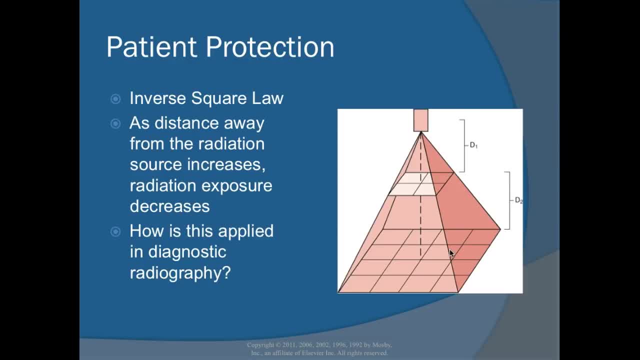 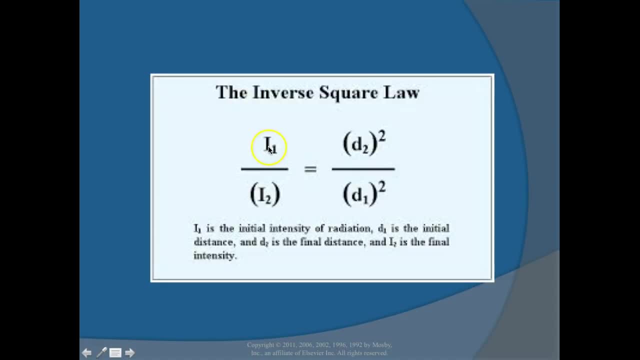 of radiation that you're getting, but the amount of radiation that you're getting. so the way that you're getting those photons, they're just spread out over a larger area. so here's your inverse square law. oh sorry, that's so fuzzy. so you have your. intensity of 1 over intensity 2 equals the distance of 2. 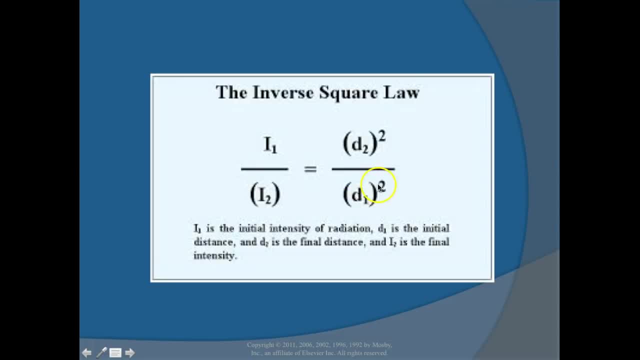 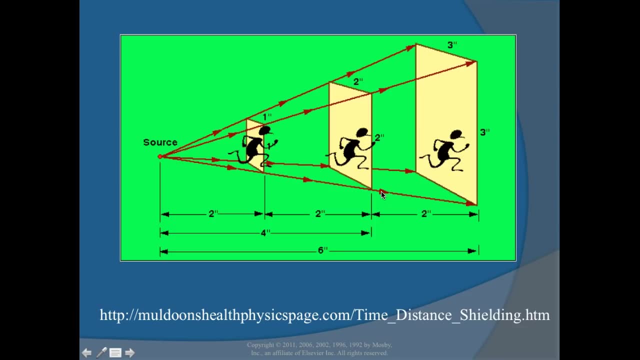 squared over the distance of 1 squared inverse, so they're inversely related squared. okay, don't forget the squared part. so, as you can see, here we have a At two feet. you can see at same size person here as you go if you double your distance. 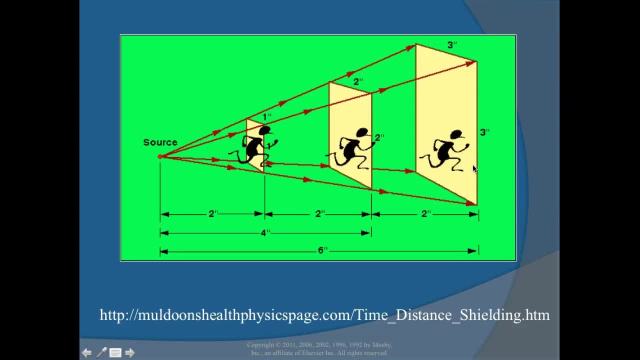 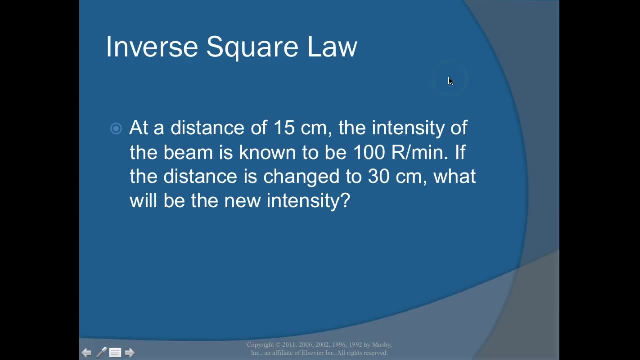 and then you take it up to six feet. you can see here that the photons are spread out over a larger area. So at a distance of 15 cm, the intensity of the beam is known to be 100 R per minute. If the distance is changed to 30 cm, what is the new intensity? 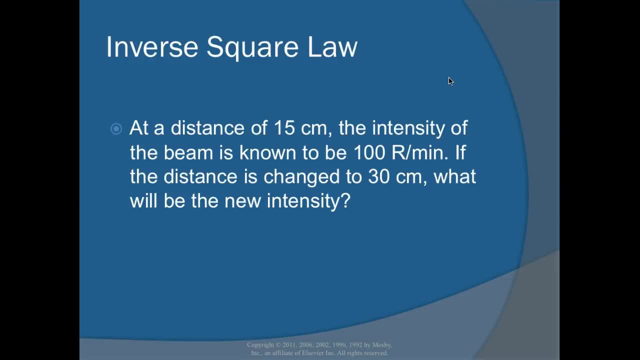 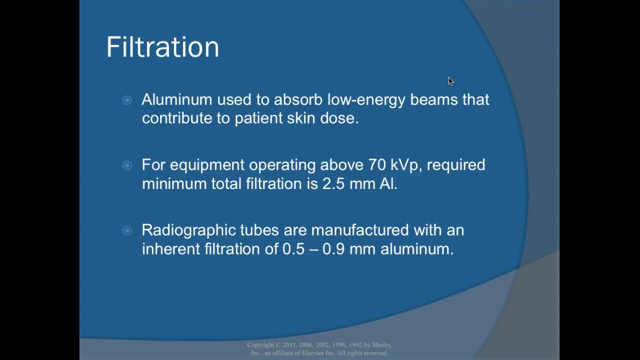 So you'd have to calculate that out. I think it's 25.. I think I'd have to calculate it out. All right, Filtration, What is it? Oh, let me just say here: be sure that you can calculate out the inverse square law. 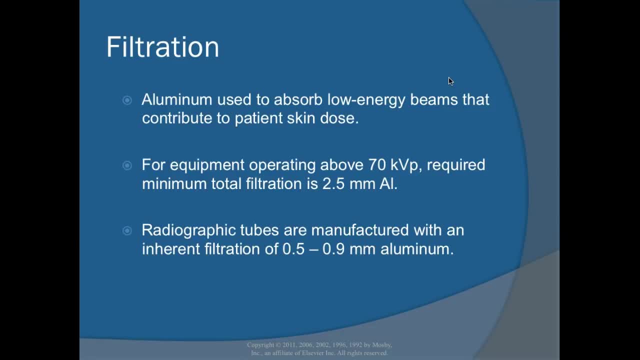 We'll all have stuff for you to practice. Okay, Filtration: It's aluminum that we use to absorb low energy X-ray beam. that contribute to patient dose, So really it's just skin dose. So these photons don't have enough energy to even penetrate past the skin. 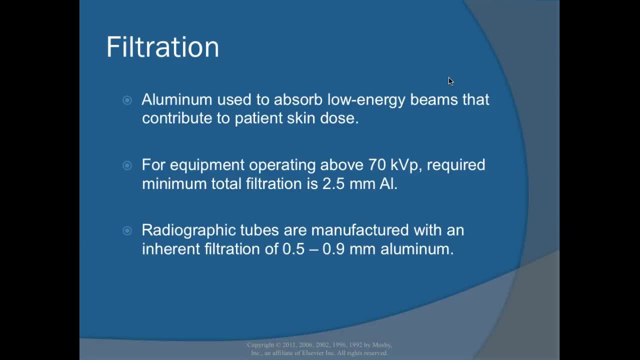 So we use filtration to filter those out. So that's what we're really talking about with our classic. Okay, So we use a filter to take out the photons that would only contribute to skin dose. For equipment operating above 70 kVp, required minimum filtration is 2.5 mm of aluminum. 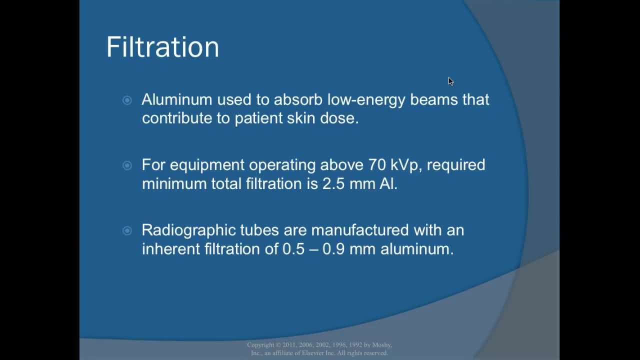 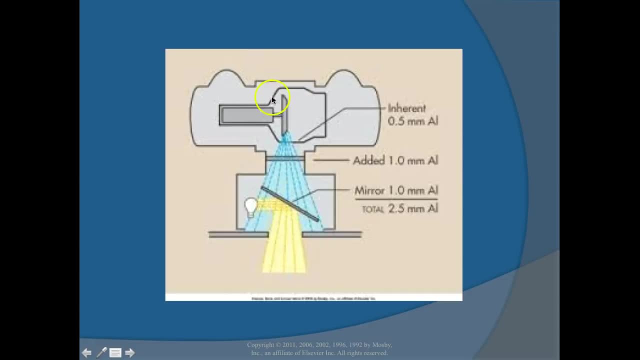 Radiographic tube. Radiographic tubes are manufactured with an inherent filtration of 0.5 to 0.9 mm of aluminum. So we're looking here. Here is our X-ray tube and you can see our glass housing, and then we have our lead housing. 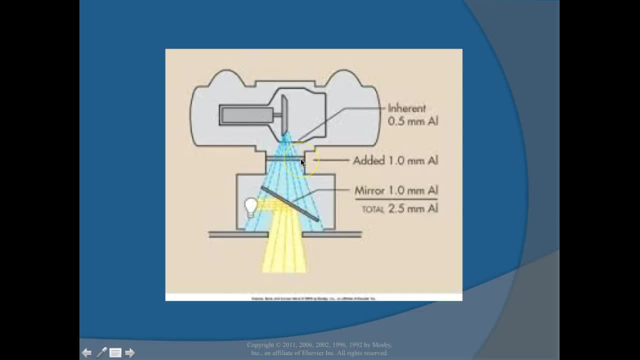 around the outside and we have 1 mm of aluminum here. Our mirror is 1 mm of aluminum and then our window coming out of our X-ray tube is 0.5 mm of aluminum. So the 0.5.. With the 1 mm plus, our mirror out of 1 mm is 2.5 mm of aluminum. 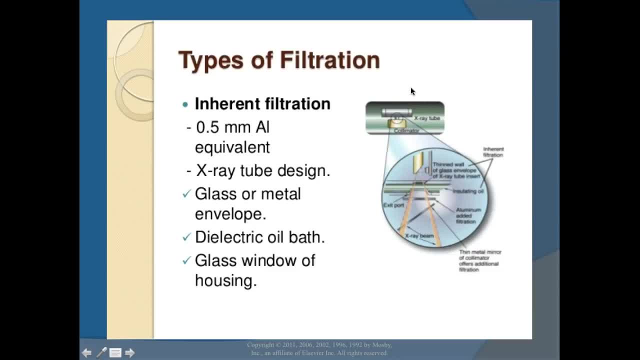 So here is out of Carlton, and this is a book that you guys will have your second year and you can see this component right here and we've got all the different filters there equaling 2.5 mm, So 0.5 mm or equivalent. 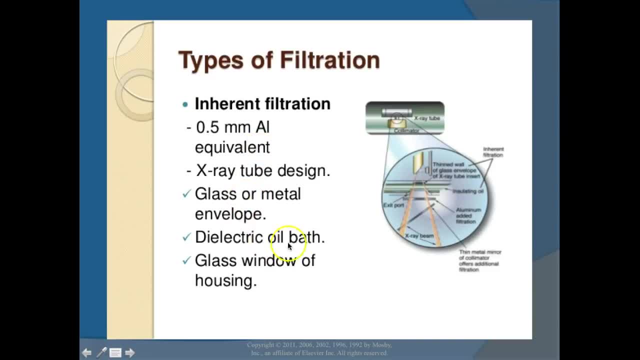 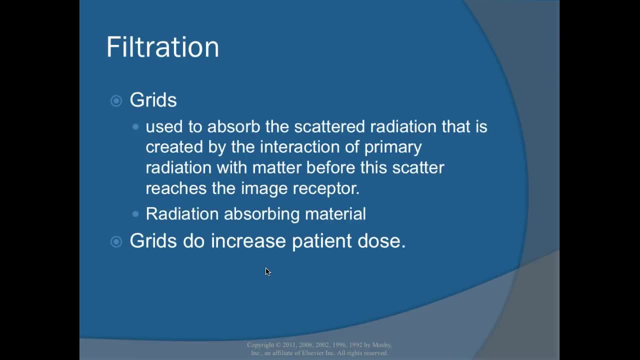 Then we have the tube design, We have the glass or envelope, We have the, The oil bath and the window for the housing. So all of it equals the point 2.5 mm of aluminum. So, grids, we use them to absorb scatter radiation that is created by the interaction. 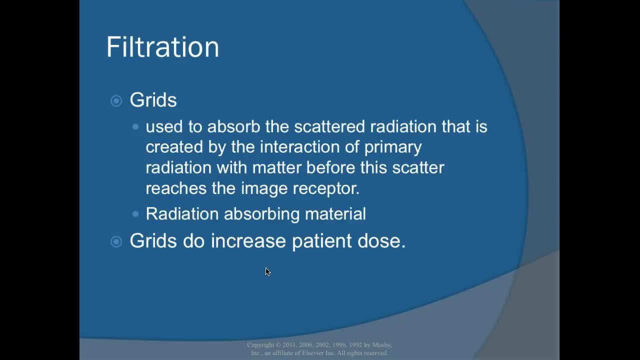 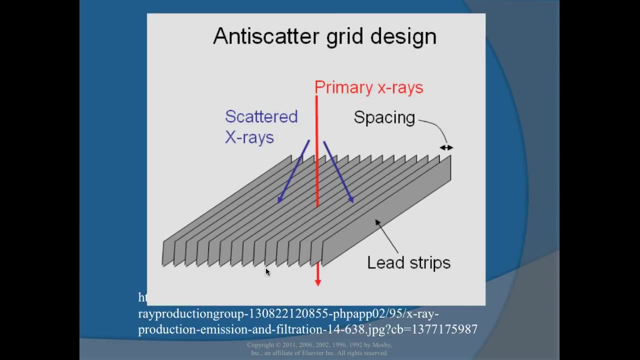 of primary radiation with matter before the scattered reaches the image receptor. So radiation absorbing material. So we use typically lead or aluminum grids. do not increase patient dose. Okay, why? because they're placed underneath the patient. so what happens is you have your primary x-rays. they're coming straight down. they are going to make it through all these. 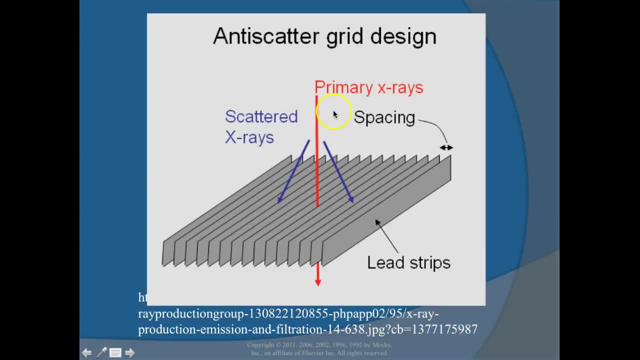 little led strips because they're going straight, but the scattered photon that's coming out of the body, going sideways here, is going to get absorbed by these led strips so that they're not getting through, because it's misinformation if this piece was representing the kidney, but it's coming off. 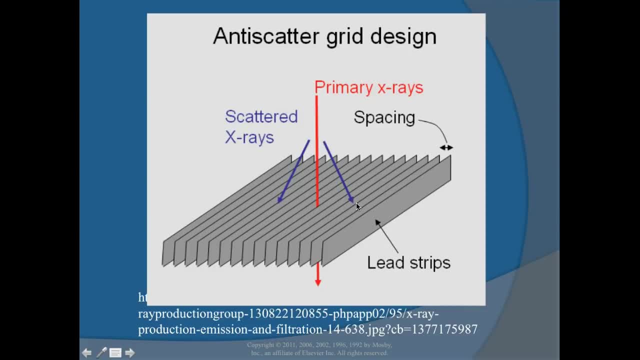 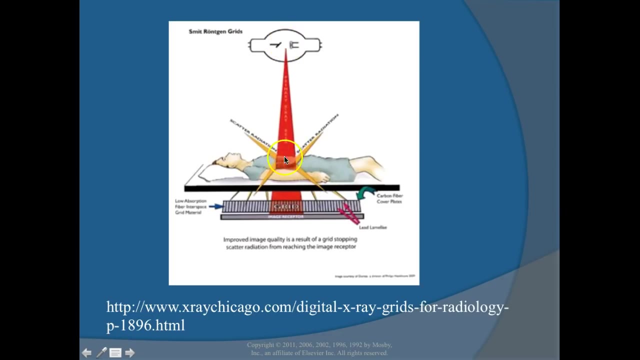 It's going to misrepresent the kidney size, shape, pathologies, everything so coming straight through are the diagnostic ones that we want. so a grid is going to clean up your scattered x-rays. So you can see, here you have your x-ray tube coming down, you have scatter radiation going. 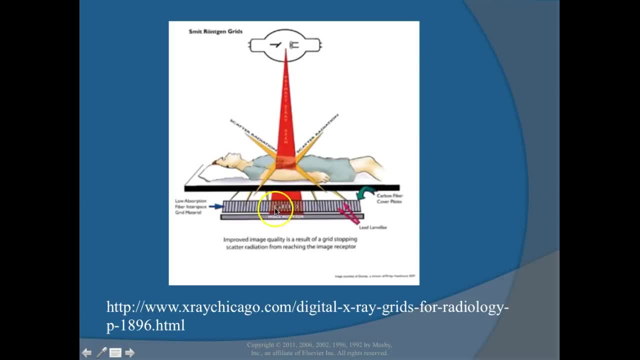 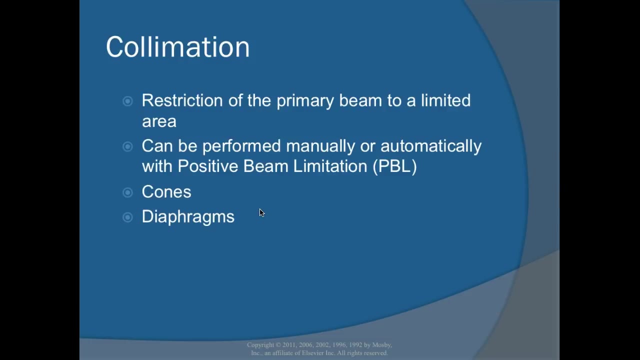 in all directions. you have a grid here and the grid is only taking the photons coming straight through to hit the image receptor, so that the grid is always underneath the patient and above your image receptor. collimation- restriction of the primary beam to a limited area can be formed manually or automatic with PBL, which is positive beam limitation, you 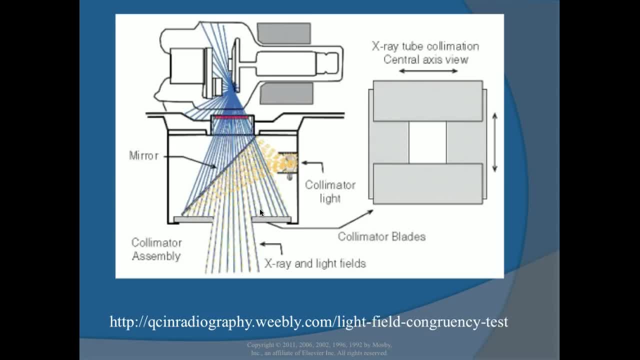 can use cones or diaphragms. we have diaphragms on all of our tubes and you can see, here we have your. here's your tube, here's your window, then you have aluminum and then we have our mirror And here's the light. this is how it works, and you have your collimators here. so here's. 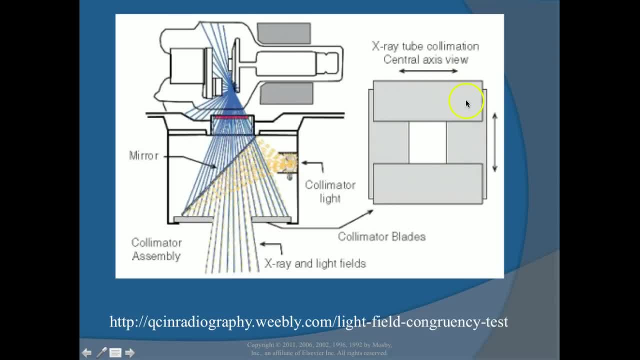 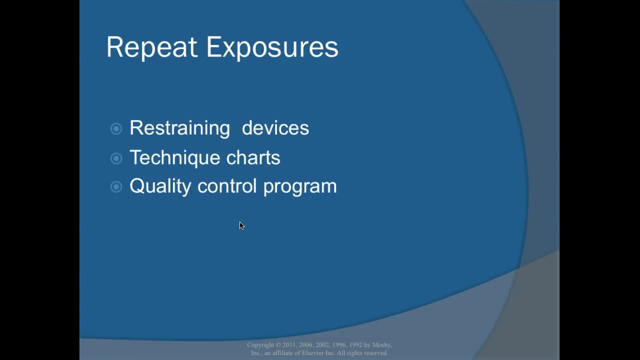 your blades you have in two different planes here. so these shutters come together this way and these guys come together this way so you're able to shrink it down to just the size that you need for the patient. Repeat exposures are really really big on patient dose, so use restraining devices, devices. 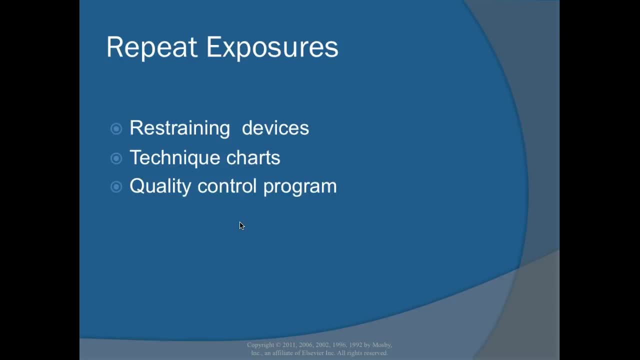 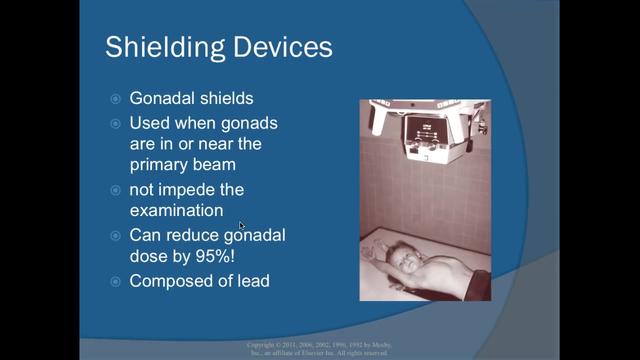 if you can Make sure you use a technique chart or know the technique for what you're shooting. don't guess. and make sure that there's a quality control program in place to make sure that, one, your repeats are within range there's and, two, there's nothing wrong with your equipment. 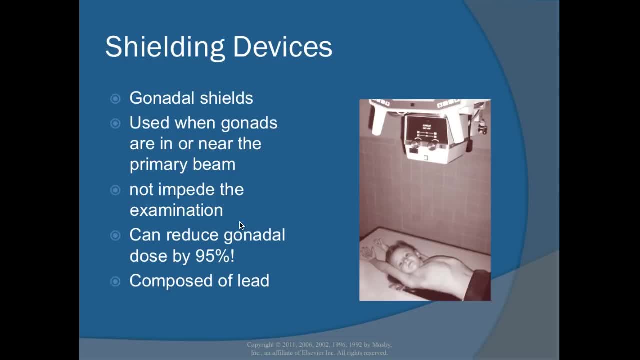 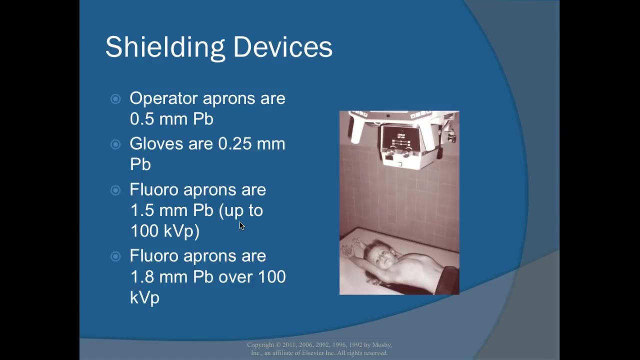 Shielding devices, so gonadal shields use when gonads are in or near the primary beam. they should not impede the exam and can reduce the gonadal dose by 95 percent. so they're composed of lead. Any kind of shields are lead, So operator aprons are point five millimeters of lead. pb means lead, pb is lead, gloves are. 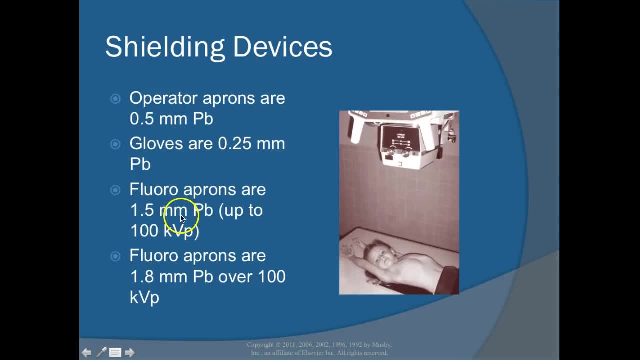 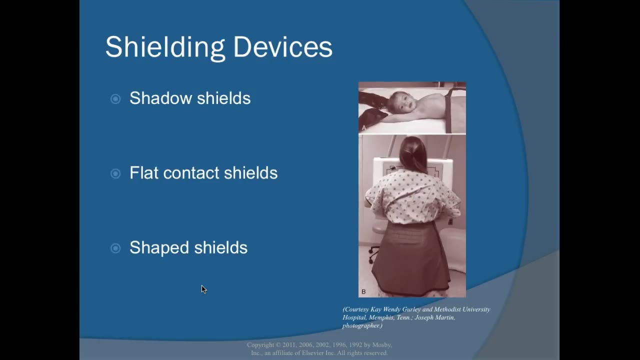 point two: five millimeters of lead. floral aprons are one point five millimeters of lead up to 100 kbp and one point eight millimeters of lead over 100 kbp. Know those numbers. There's different shielding devices, So there's shadow shields, flat contact shield and shape shields that we use for patients. 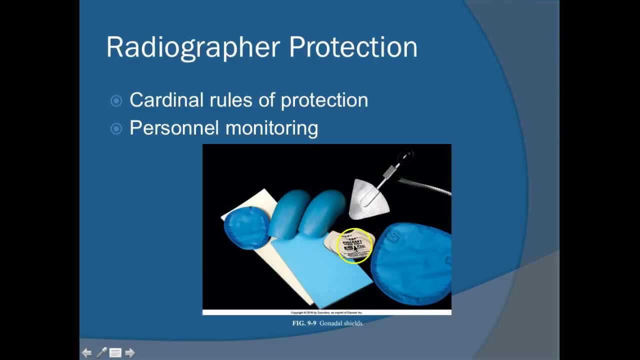 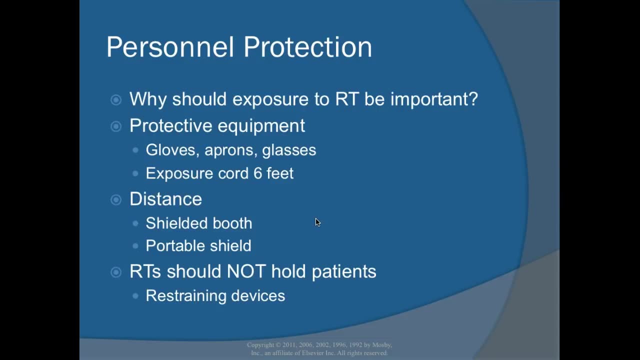 and here's some of them. You can see these are just little flat contact shaped, So give you an idea. the different ones. All right, Personnel protection. Why should the exposure to an RT be important? So we don't want to expose you. 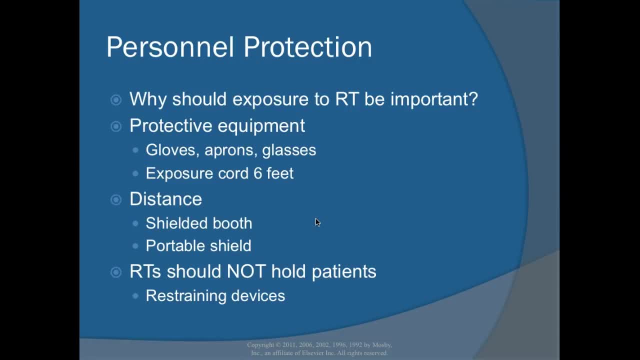 You are not allowed to hold as a student, as you know. So protective equipment: we supply gloves, aprons and glasses, and the exposure cord on a portable should be six feet. In the diagnostic rooms, the exposure switch needs to be zip tied to the console so you 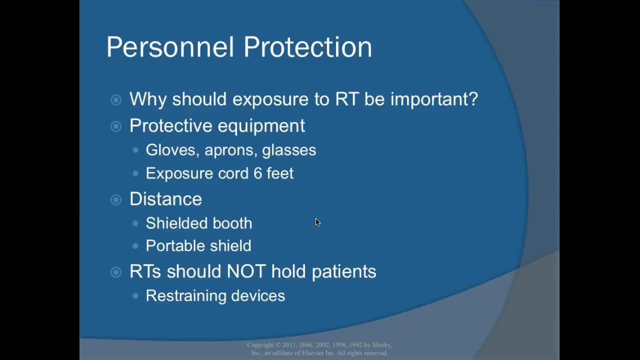 cannot walk around the corner and expose All right. So distance is your friend. You need to get behind a shielded booth or a portable shield, and RT should not hold patients. Try to get family members to hold the patient or use restraining devices. but as a student, 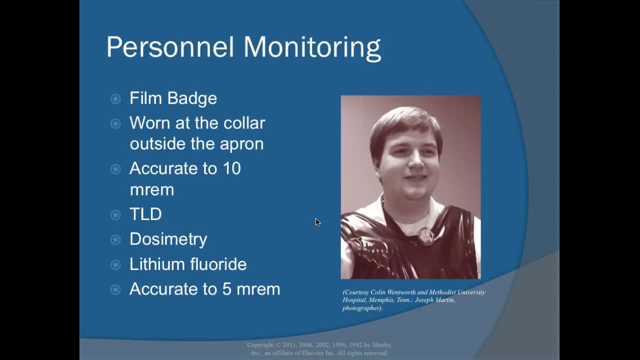 you are flat out not allowed to hold All right Personal monitoring. So film badge worn at the level of the collar, outside the apron. It's accurate to 10 milli rem. There's TLD dosimetry- lithofluoride, and it's accurate to 5 milli rem. 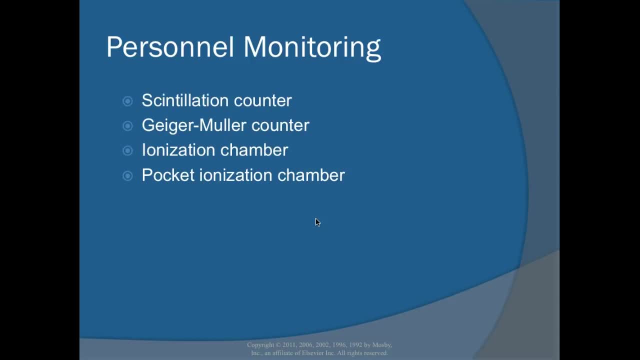 All right, So personal monitoring. There's a scintillation counter, a Geiger-Muller counter, an ionization chamber and a pocket ionization chamber. So we have: We have Geiger counters, we have an ionization chamber and we do have packet ionization chambers. 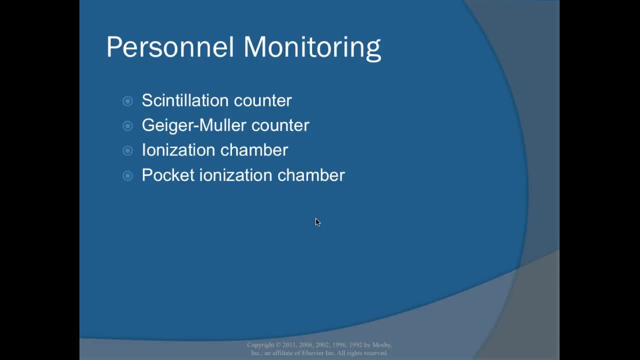 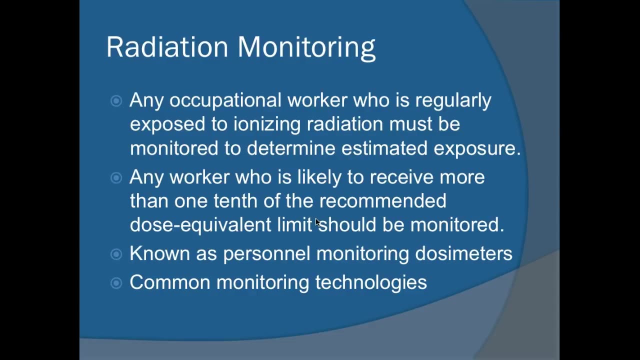 but I have not figured them out to be accurate. They work about half the time. All right. Radiation monitoring. Any occupational worker who is regularly exposed to ionizing radiation must be monitored and determined estimate exposure: Any worker who is likely to receive more than one tenth of the recommended dose equivalent. 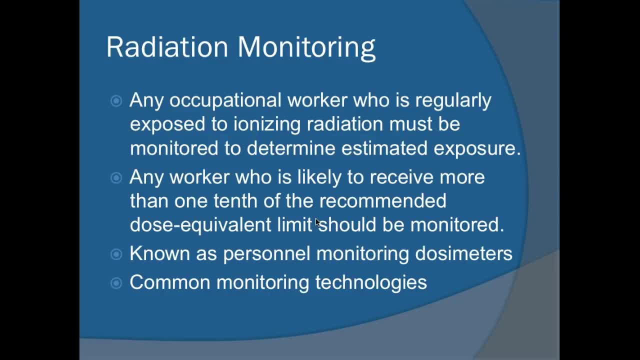 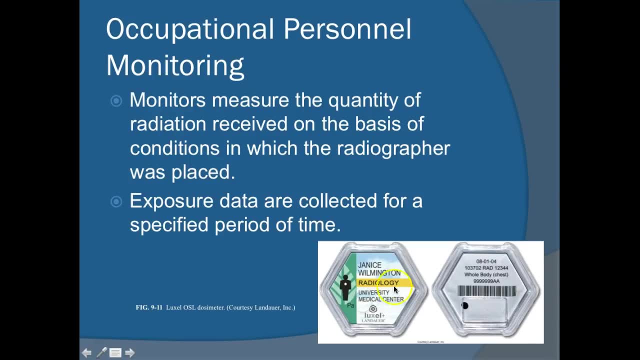 limit should be monitored. So It's personal monitoring dosimeters. It's common monitoring technologies, like you guys have those little blue jump drives, That's what those are. We used to have this here, Landauer, and it was a disaster for us.